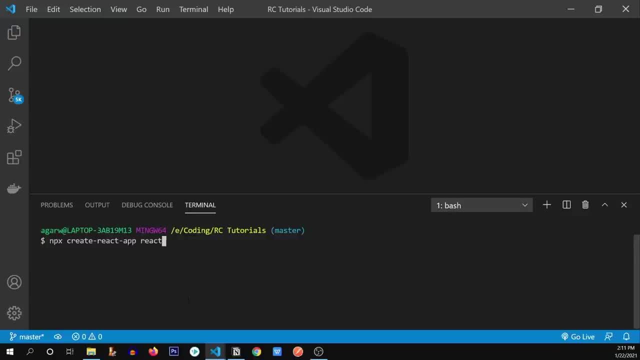 and the name of our app, which I'm going to give React Router tutorial. Now, what it's going to do? it's going to go to NPM website or NPM repository. I'm going to take all of the things needed to create a new React app And it's going to put all 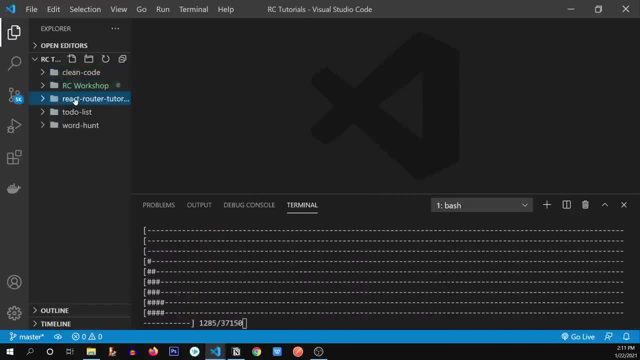 of those things into this folder react router tutorial. it's going to find all of the dependencies that we need to create our React app And it's going to basically initialize a boilerplate code for our React app. Alright, so it has successfully initialized our new React app. 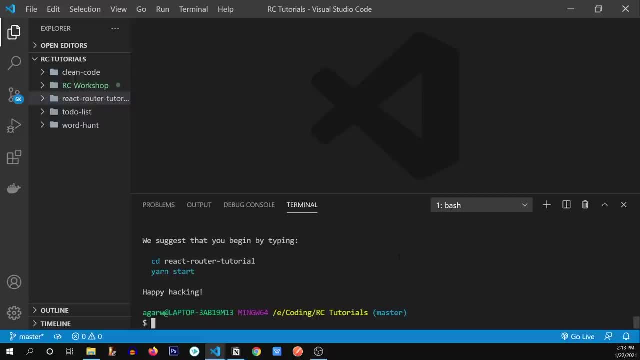 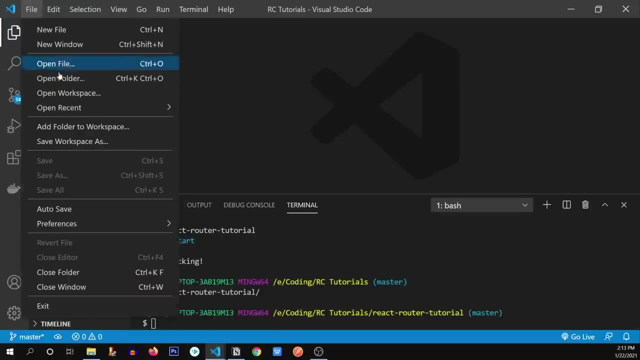 Now we need to switch to that folder. what we can do is either we can type- we can type cd and the name of the folder. you can switch this way- Or what you can do is you can open that folder in VS code, which in my case is this folder, And I'm going to select this. 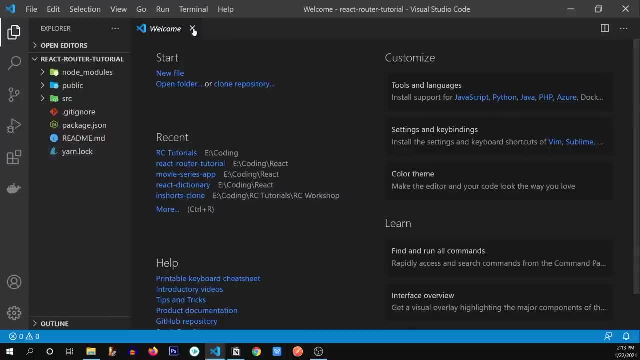 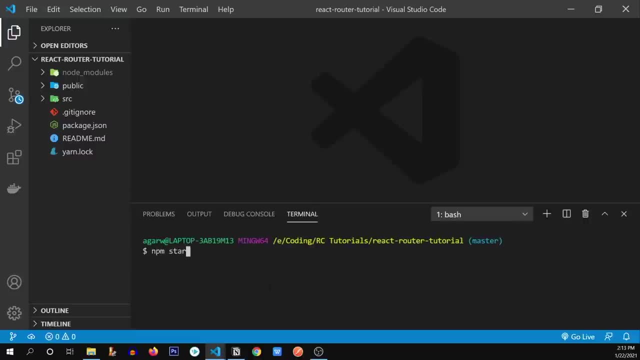 folder. So here we go. our folder has been opened in the VS code successfully, So what I'm going to do now is I'm going to type npm- start. So it's going to start our React app. Here's our React app running successfully. 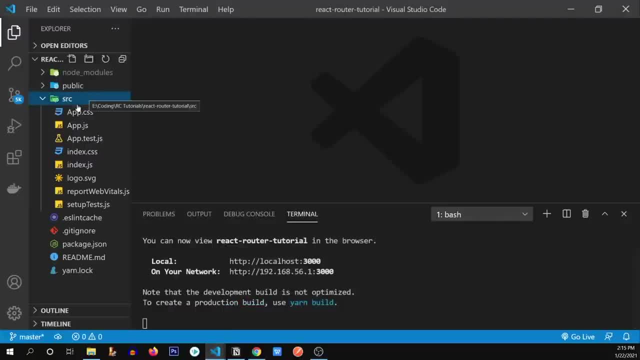 So what I'm going to do now is I'm going to go, I'm going to go to the SRC folder And I'm going to get rid of those things that we don't need. So this, this, this and this, we're going to get rid. 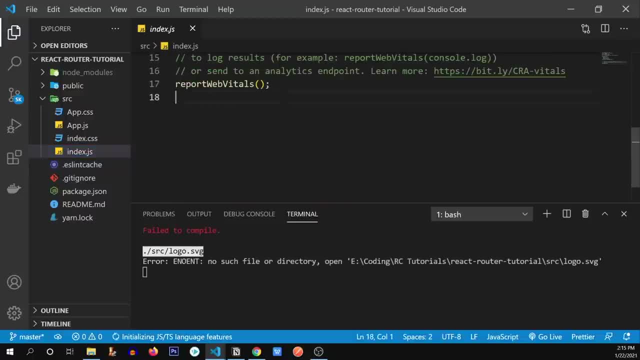 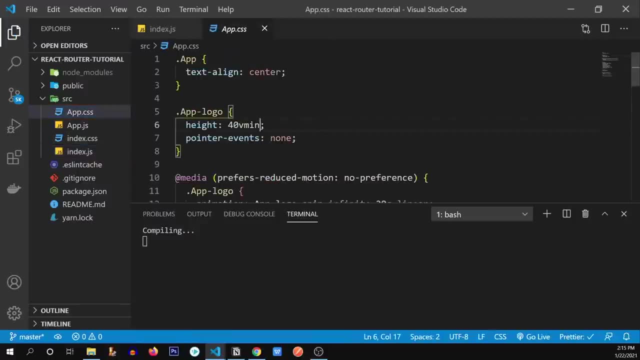 of these four files And we're going to remove the places that they were being used. So, over here, And I'm going to get rid of all of these styles Inside appjs, appjs. I'm going to get rid of this. Get rid of logo. 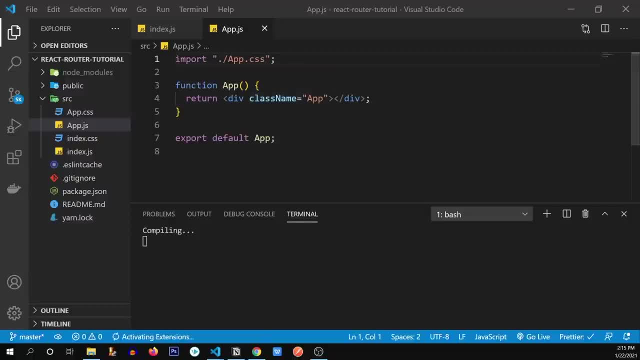 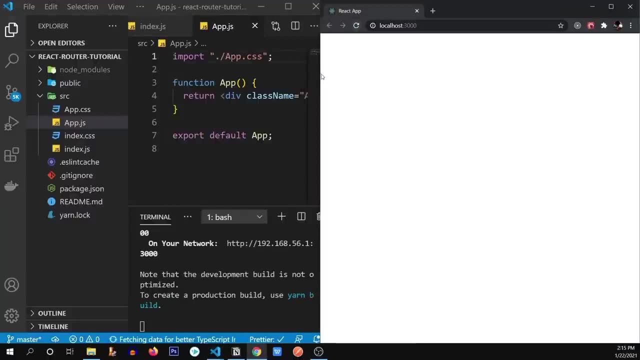 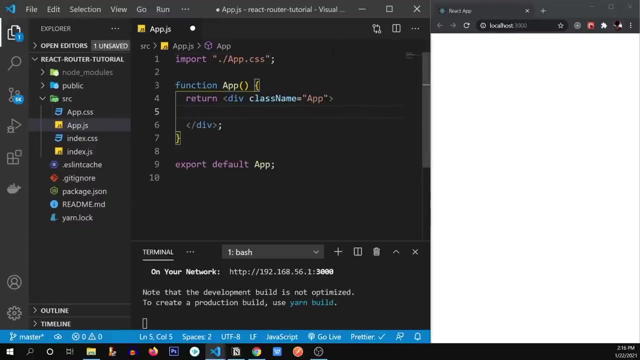 And now you'll see that our app will have nothing to show. Let me refresh it. Yeah, there you go, It's an empty page. Okay, so what I'll do now is I'm going to type h1, h1- react router DOM tutorial, or just react router tutorial. 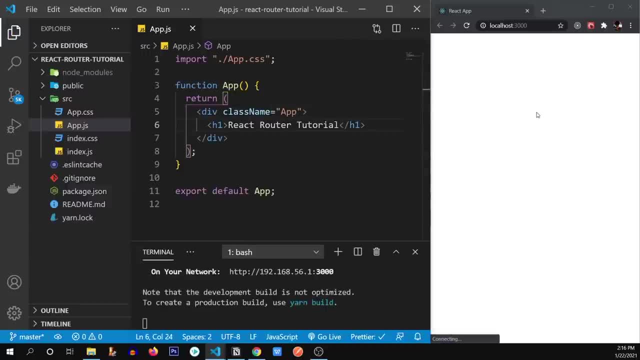 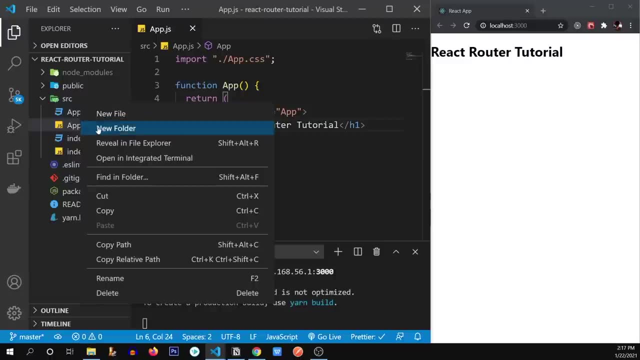 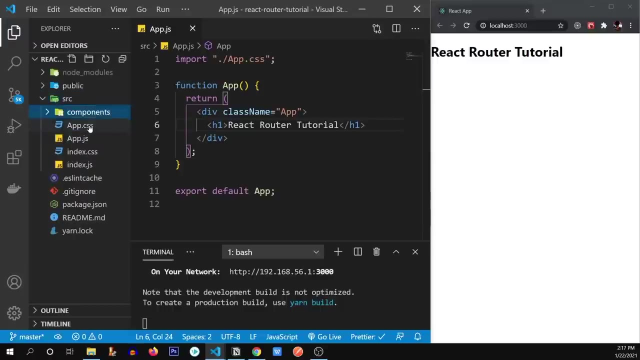 Let's save this and see: Yes, it has successfully rendered this over here, So let's create a different component for header. I'm going to create a new component called I mean- new folder called components. It's not necessary to create a separate folder for components, but it's a good practice. 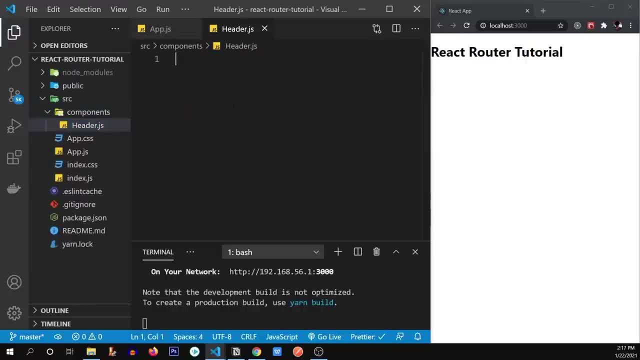 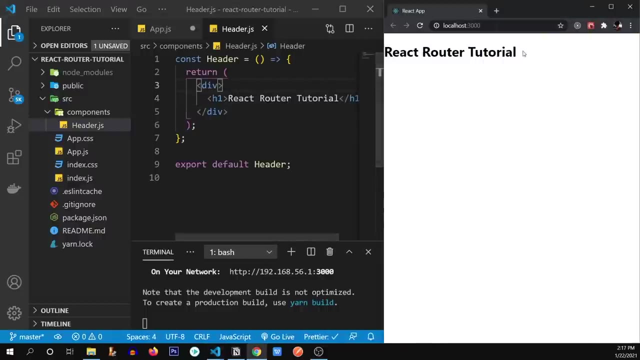 I'm going to create a different component for header dot j s And I'm going to type r a f c e, underscore r a f, c, e, And press Enter And let's copy the same thing over here. Here we go. Let's first center align this thing, And then we're going to start with our tutorial. 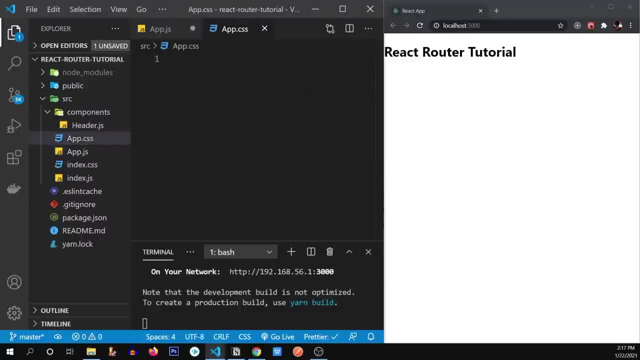 So I'm going to give it a few of the styles in app dot css. I'm going to give it a display flex And justify content. No, sorry, I mean to say align Items to center and flex direction is going to be column, because we want everything to be top down. 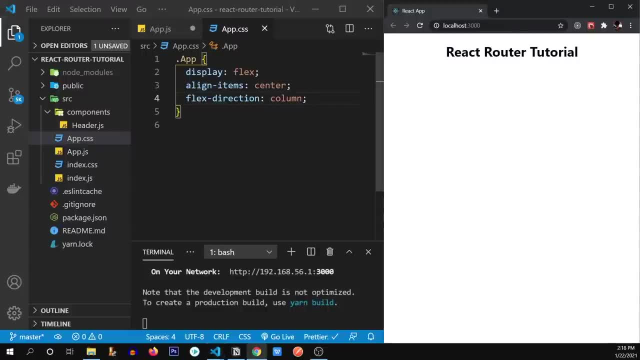 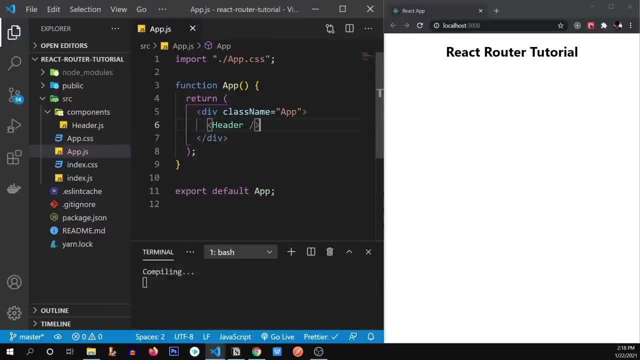 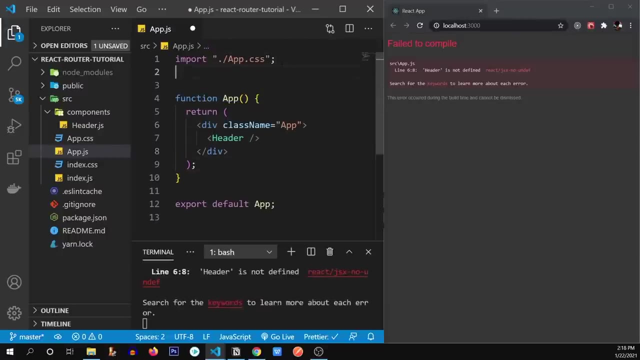 You know aligned. So yeah, here we go. It has. it is in the center. So yeah, I haven't done this, imported the header component. Yeah, Header is not defined, Let's just import it manually. So I'm just going to call this one here. 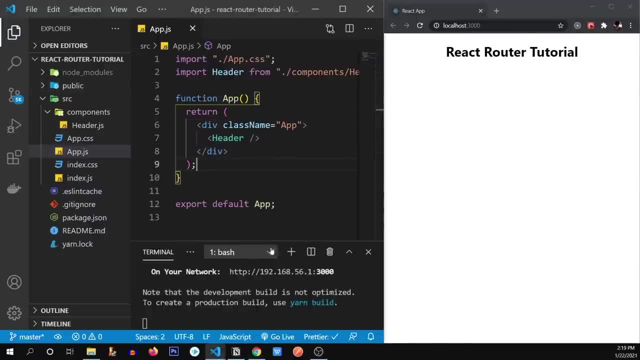 Here we go, It should work fine. Now, Yep, here we go, It's working fine. So now we are going to install a React router DOM. So I'm going to open a new terminal and type np m I- React router. And you know what I'm going to go to header and get rid of this dev. Let's use the react. 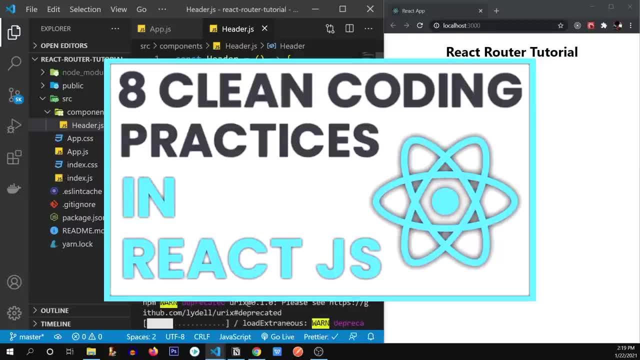 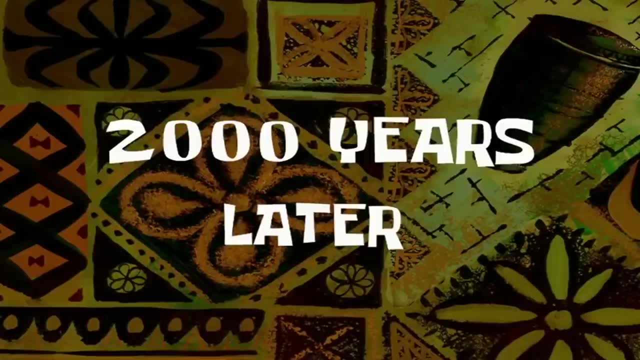 fragments. So if you don't know what react fragment is, you can watch my previous video on 18 code practices in react. it's going to help you a lot 2000 years later. or it's a: finally, a react router DOM has installed successfully, So I'm going to go to my app. 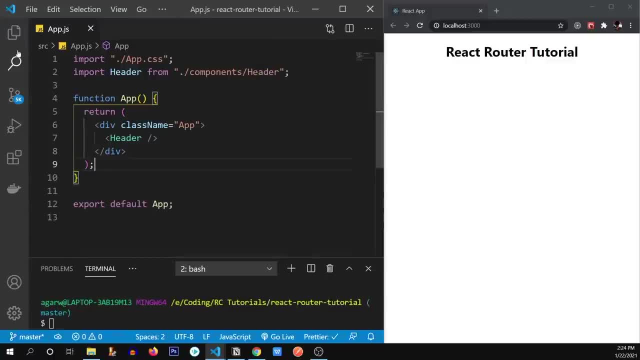 JS component And to use our react router DOM. what we'll need to do is we're going to have to cover this whole react app in something called browser router- browser router- which comes from react router DOM. So you can see, it has auto imported, So I'm going to wrap. 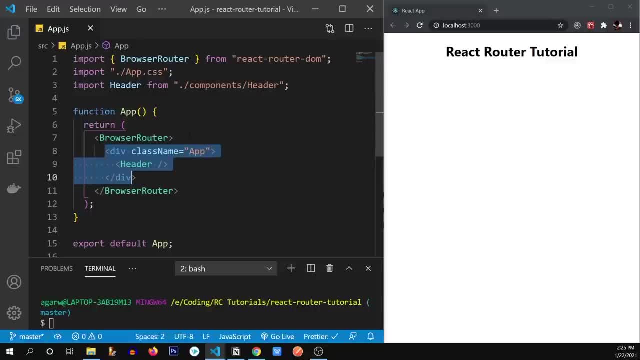 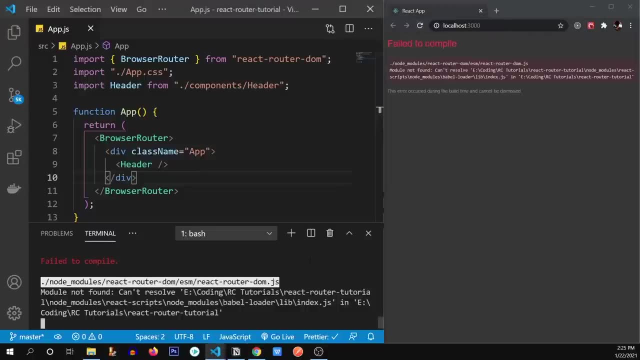 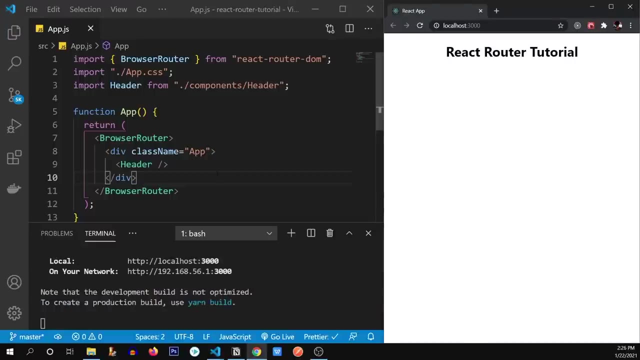 whole of my app in this. Alright, here we go. Let's close this terminal. I think I'm going to have to restart my application, So let me just do that quickly. Alright, it's fine now. So what are we going to do next is we're going to create different, different. 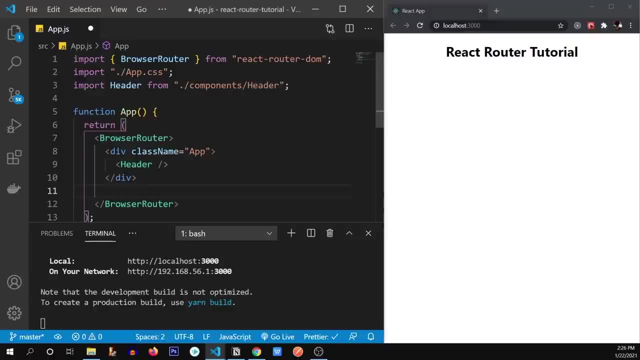 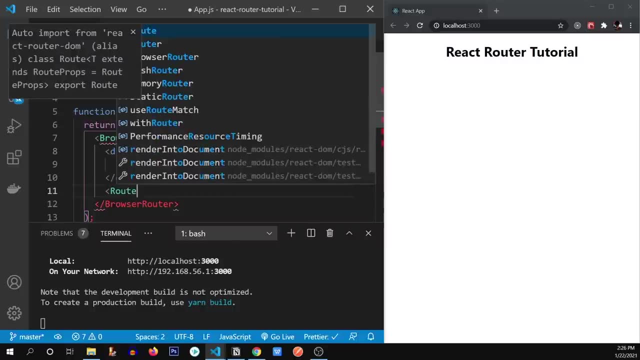 routes for different different pages that we're going to work with. So let's create our out for homepage, about page and profile page. Yeah, So I'm going to type route and press Enter And you can see route has auto imported from VS code, I mean from React. 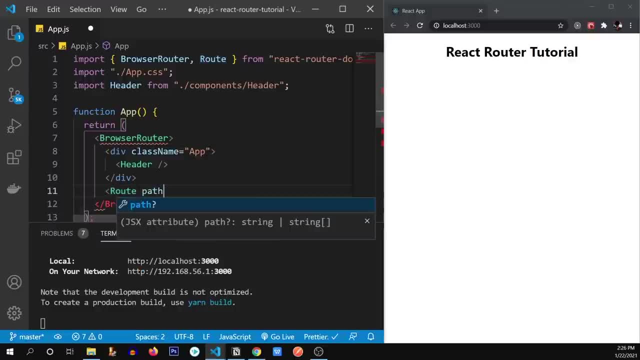 router. DOM VS code has auto imported it, So I'm going to give it a path. This is going to be a home page, So it's going to be this. have to give it a component which we'll create in a second, So let's duplicate these paths. 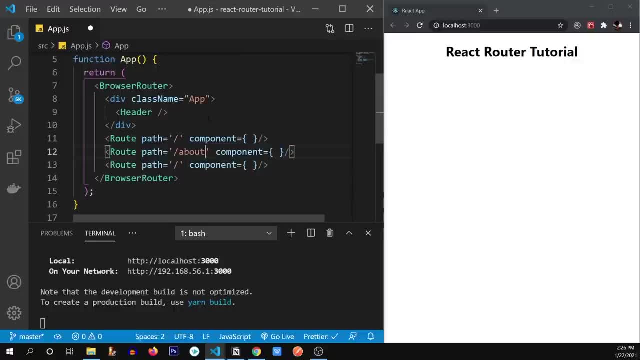 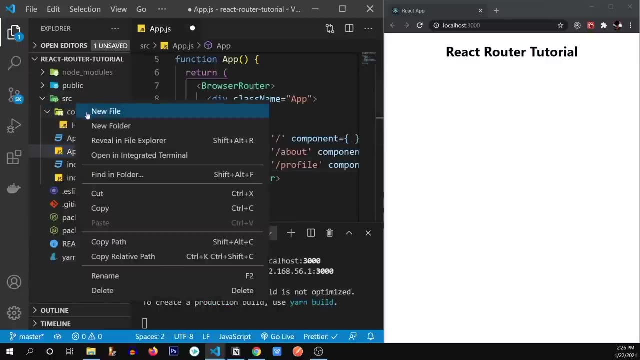 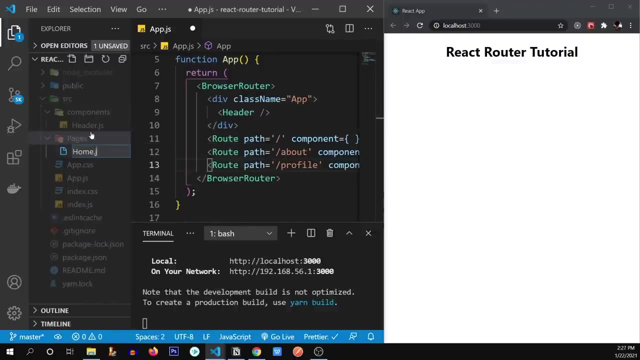 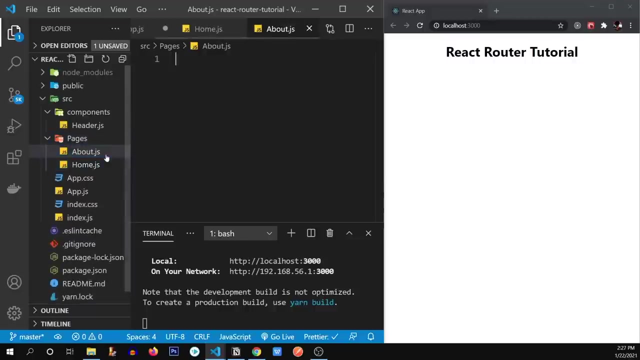 Another one will be for about and the third one will be for profile. So let's create these pages. First, I'm going to create a new folder with the name of pages, homejs. I'm going to get another file called aboutjs, And the third file will be profilejs. 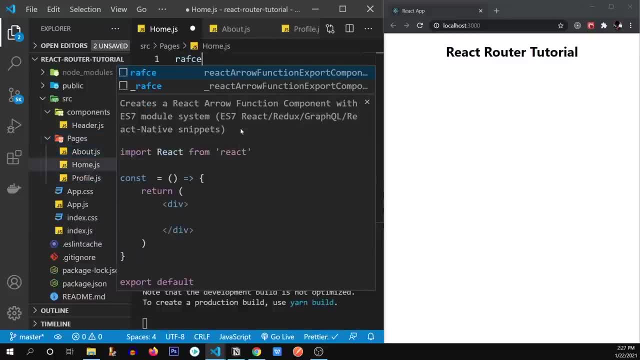 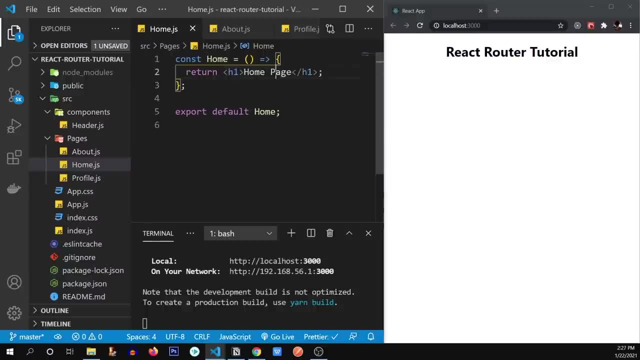 Let's let me quickly write some code inside of this. Let me type home page, remove these divs and add h1. That's better. Same thing with the aboutjs page- About page- and the profile page- All right, cool. Profile page- All right, cool. So we have created all of our three. 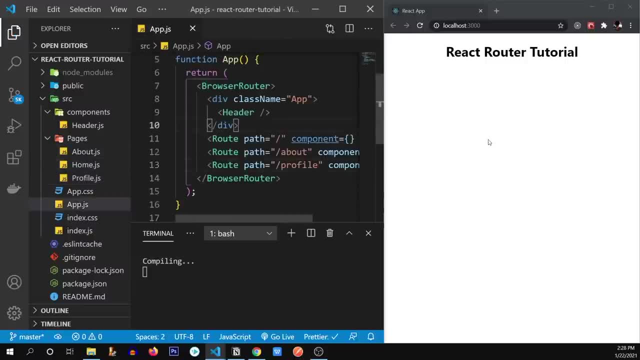 routes. Now let's test these routes, if these are working or not. So let me save my app real quick. Okay, there's an error. What's the error? Okay, we haven't given an error. We haven't given an error, So we'll give an error. 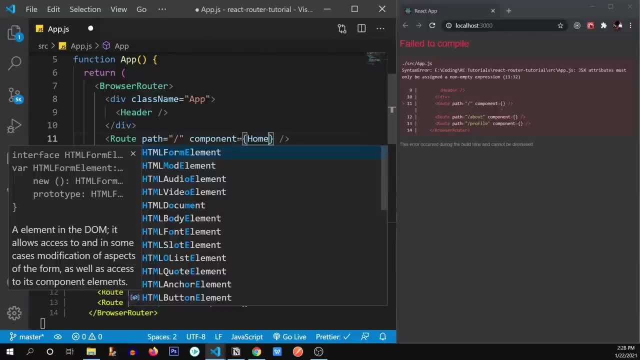 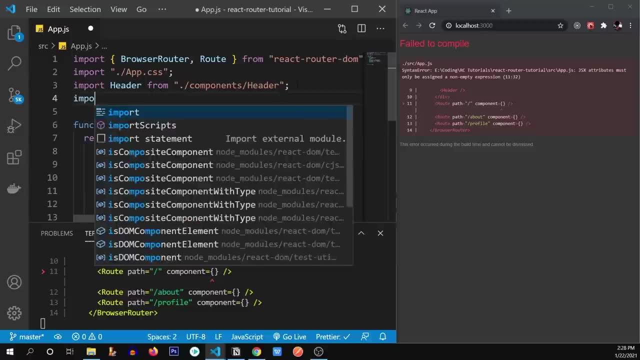 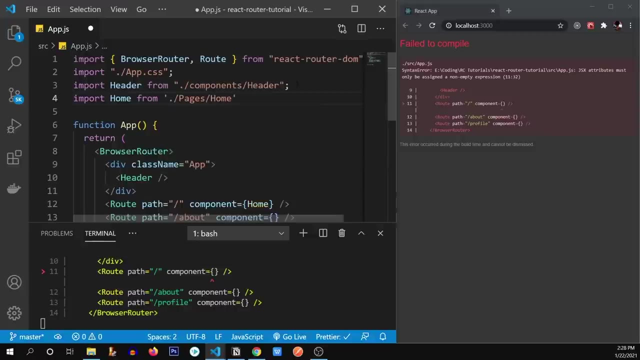 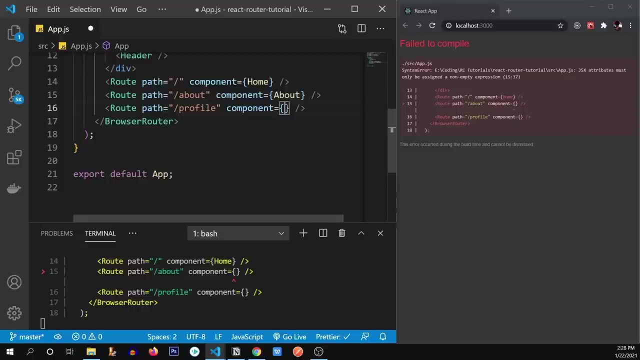 the components, obviously. So let's just give this home door. Oh, sorry, My bad, We have to import all of these components first. So import home from slash home and I'm going to do for about and profile as well. So about and profile. Let me just about and profile. Here we go, So we 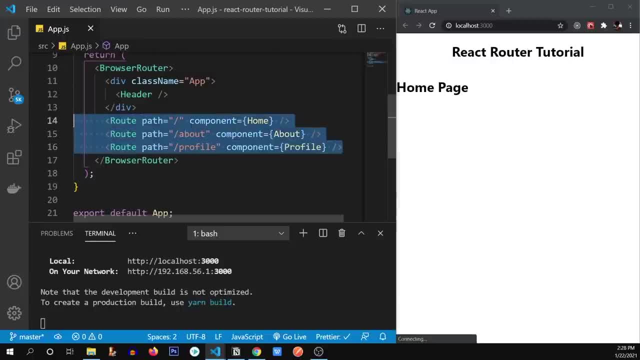 have created three routes. This is how you create routes in react by using react autodom. So you can see it's currently in the root folder, I mean in the root path. So it's giving us homepage. Let's go to the about page. 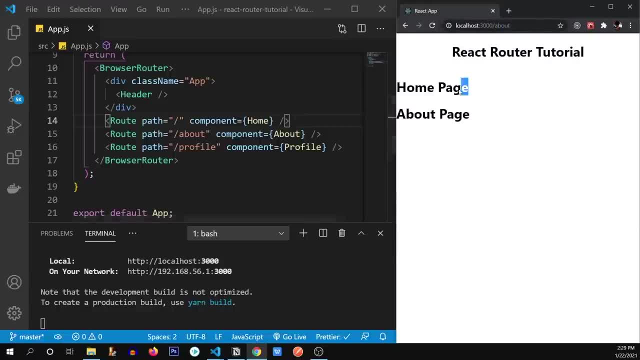 About. here we go, it's giving us about, but you can see the homepage is also appearing here and about pages also appearing here. Why is that happening? Because you can see it. it has about page as well And this route as well. In this, in its path, it has route as well. So what we can do: 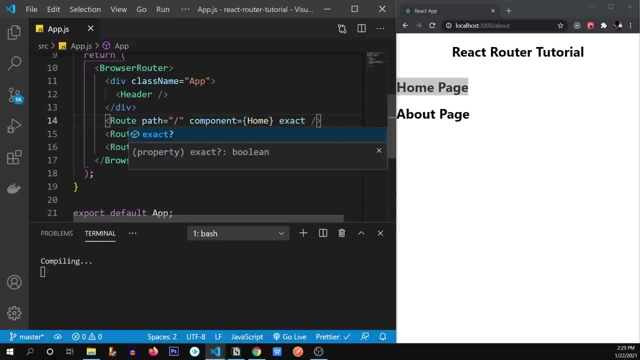 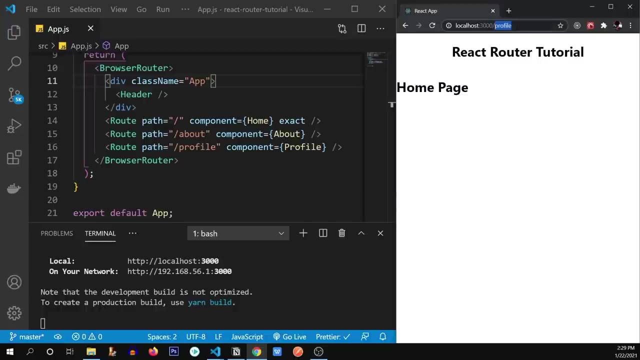 is we can type exact, So it's going to go exactly to this path and not nowhere else. So if it out type about, it's going to clear, open about page And if you type profile, it's going to go to work. 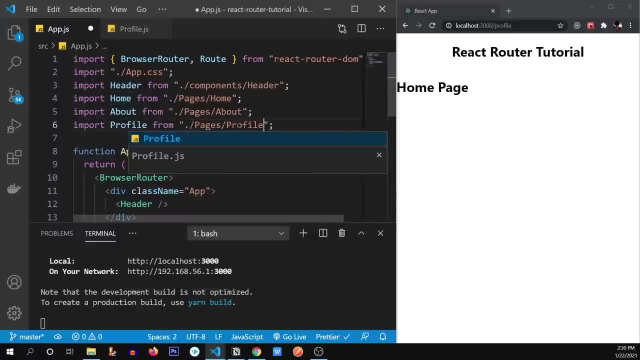 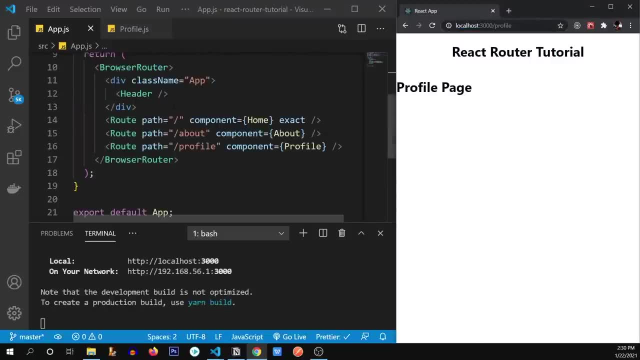 Okay, I have made this mistake. Yeah, now it's going to work. fine, If I go to profile page, it's going to open the profile page. Another thing which you can do, apart from exact, is you can use something called switch. So if I type switch over here and I'm going to take all of 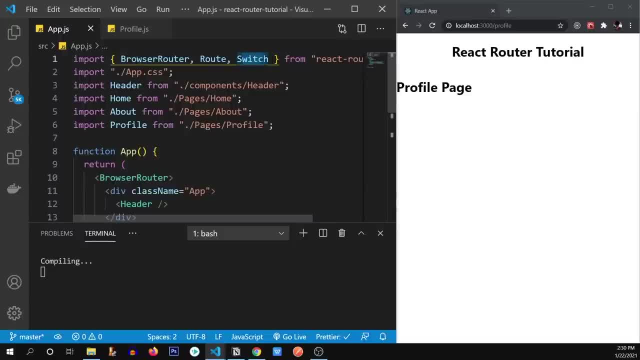 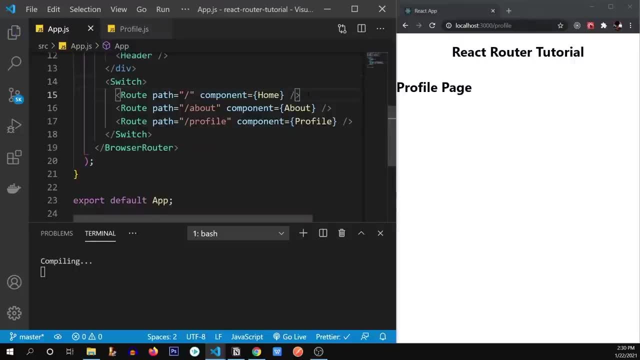 the inside of the switch and I've imported the switch from react router DOM. So what switch does is when you go to a particular path. let me remove this exact from here. So it's going to find whatever it finds first is going to stop there. For example, it has written slash profile, So it 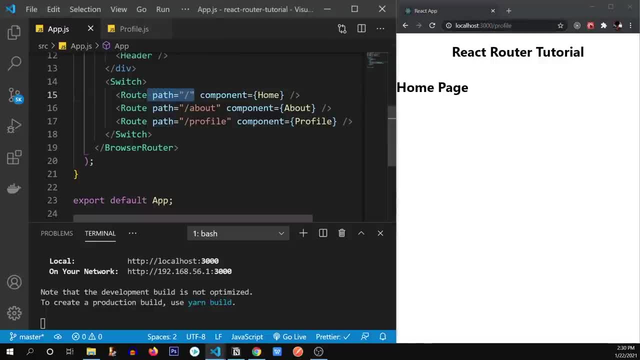 has found the slash path first. it has matched this path slash with this, So it is found. the homepage is going to render if we use switch, But if we type exact, then we're not going to have the same problem. Now You can see it's rendering the profile Now. 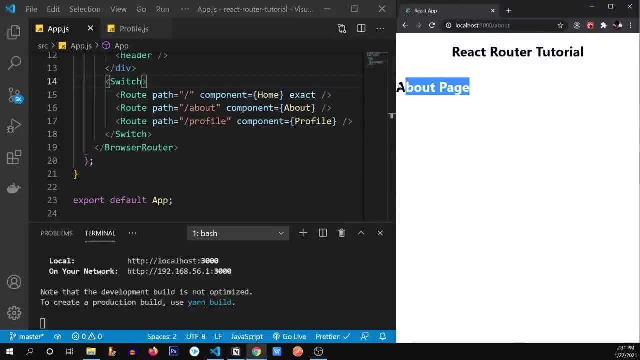 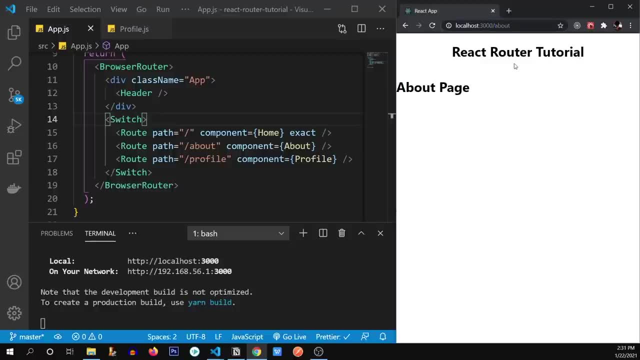 let me type about Here. we go about pitch Alright. one more thing. So we don't need to manually type this in the URL. So what can we do to go to another page? In the traditional web development, in the HTML we use something called a tag. 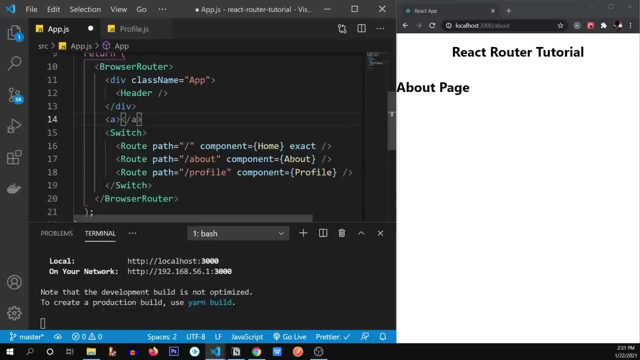 to go to a different page, So we can use that over here as well, But it has a disadvantage. What disadvantage is There? when we click on this a tag, it's going to refresh our page. Let me demonstrate that thing. 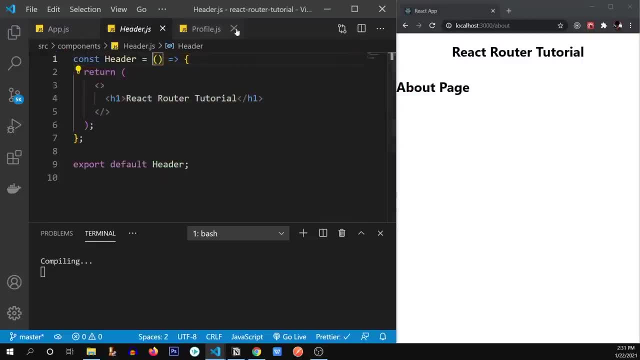 So I'm going to go to our header. I'm going to create navigation menu for our app. Let me create an unordered list over here. I'm going to create few list items and have an a tag inside of it with h, ref of no. first is going. 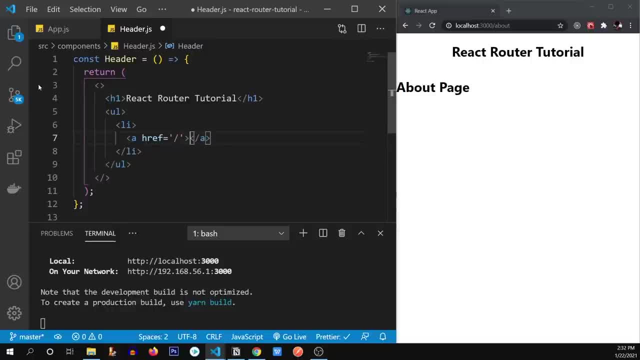 to be the homepage, So let's type slash over here and give it a name of home. Alright, so I'm going to duplicate these multiple times And I'm going to give this about about same thing here: profile and profile. Let's save this And currently looks a bit ugly, So I'm going to give it a little bit of styling. 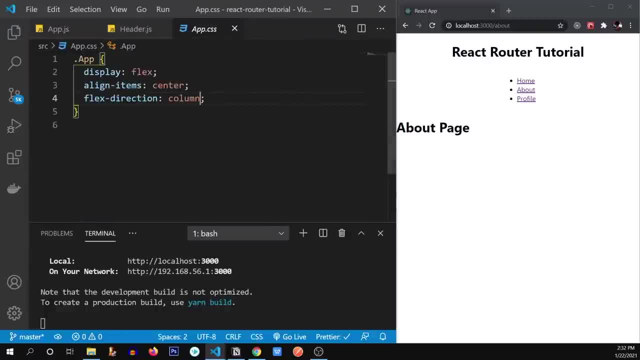 So let's go to our app CSS, And I'm going to add some styling to it. Let me give this a class name First. I'm going to give this class name of now. Yeah, Let's give it some styles. So I'm going to type list. style type is going to be none, so that it doesn't. 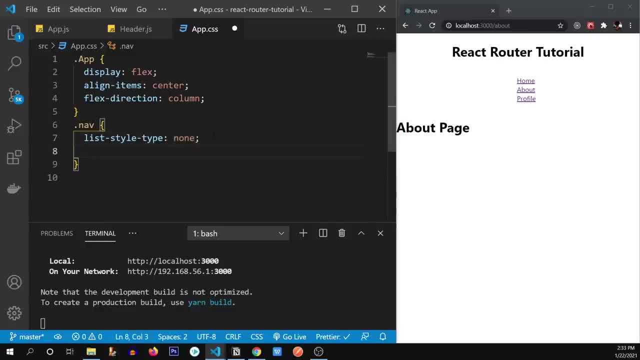 display the bullet And I'm going to type width to be 500 pixels. So I'm going to type display flex and justify content to be space evenly, so that it spreads around evenly. Now you'll see, Yep, it has spread around evenly. Now let's click on one of these links. If I'm going to click on, 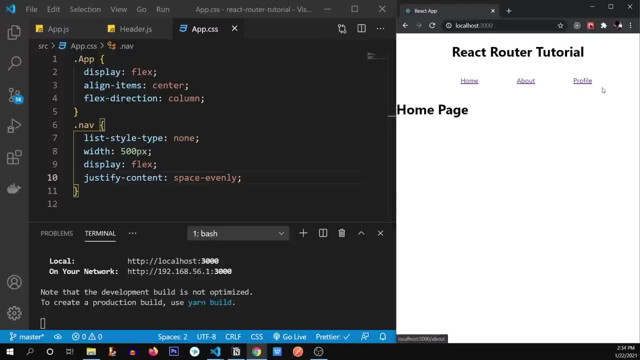 home. you can see the page has refreshed over here If I click on profile again. the page has refreshed. we've reached the destination, but the page has refreshed. we don't want the page to be refreshed. we don't want our components to. 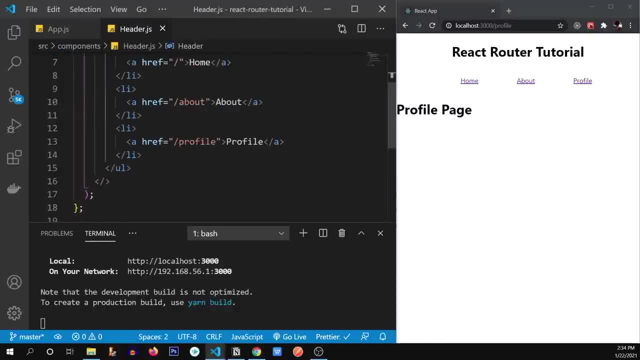 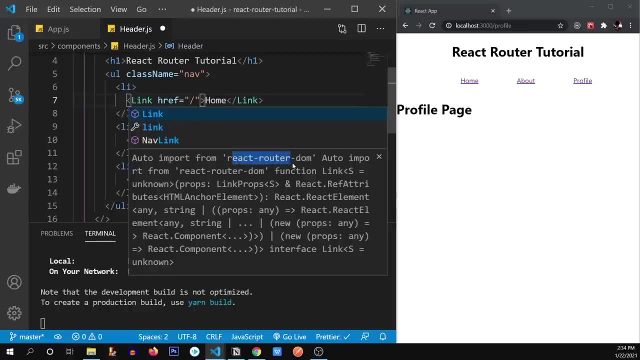 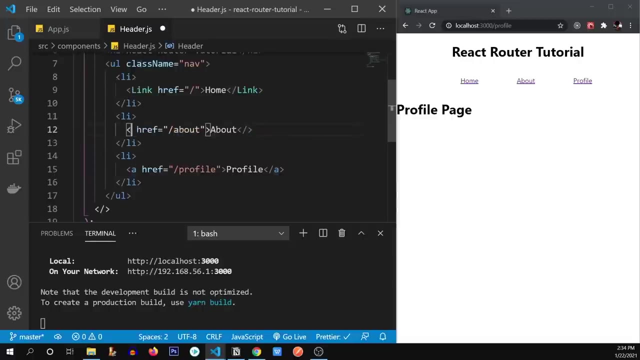 be rendered. So what are we going to do now? So instead of this a tag, what I'm going to do is I will use something called link, which is provided to us by react router DOM. Let's click on this link And you can see it has auto imported. So over here as well. Link. 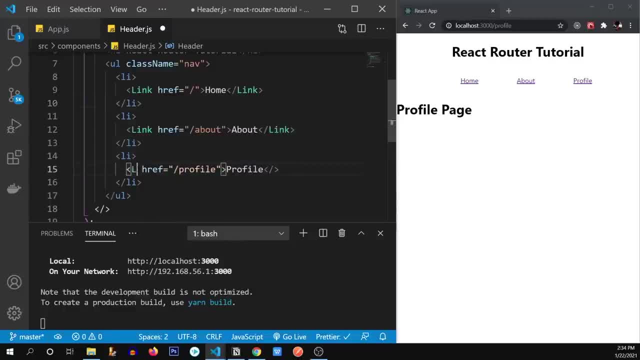 and lastly, yeah, But we can't use href with the link. we need to use something called to. this is the prop that it takes, So let's save it. All right? our app has reloaded And let's click on about Now. you can see the page has not refreshed If I click on home again. 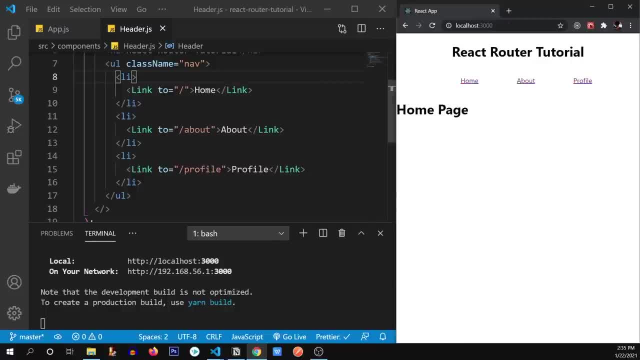 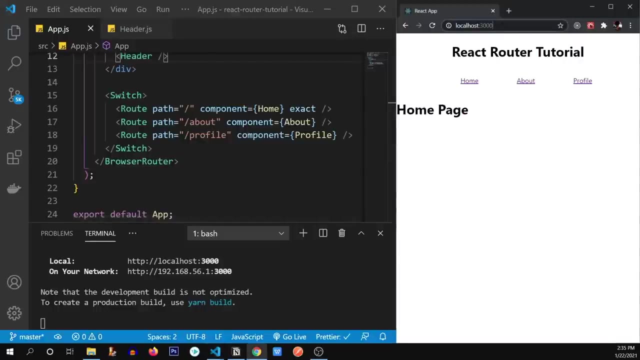 so you see, this is the power of react router DOM. it doesn't refresh your page and it takes you to another page in a blink of an eye. All right, cool. So let's discuss some more features of this library. So let's say, if I want a default route for our app, what I mean by that is: let me. 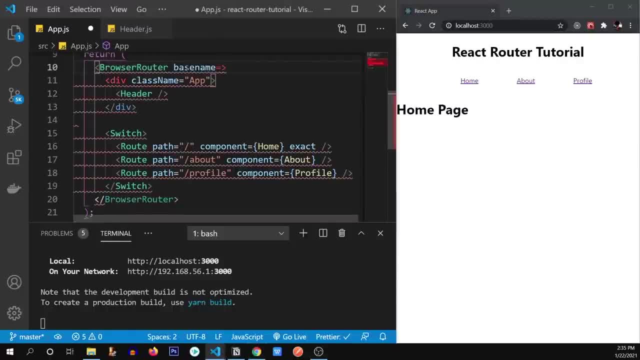 give a base name over here, If I give the base name as a tutorial and save this now you see, if I click on homepage, it's going to take us to the slash tutorial. If I click on about, it's going to take a slash tutorial, slash about. So this is how you can define a base. 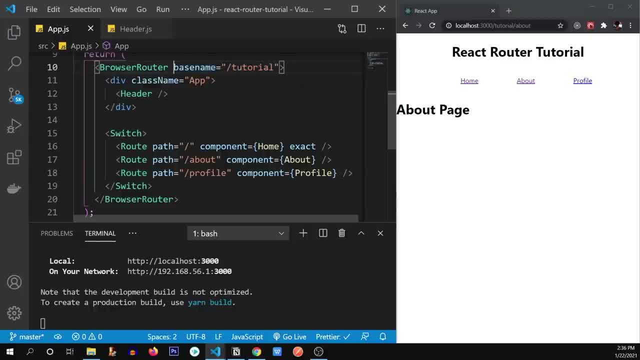 name for this by typing base name equals whatever the name that you need to use. If I click on profile, it's going to take a slash tutorial- slash profile. So this is a really powerful feature. Let's check out another feature of the browser: router. I'm going to remove this. 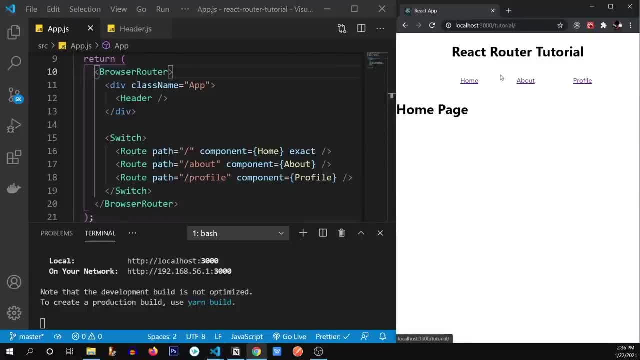 And let's say, for some reason you need to use the refresh feature. So currently it's not refreshing our page when I'm taking it to another route. So if I type force refresh over here, then you'll see what it does. If I'm going to go to about, you can see the page is refreshing. 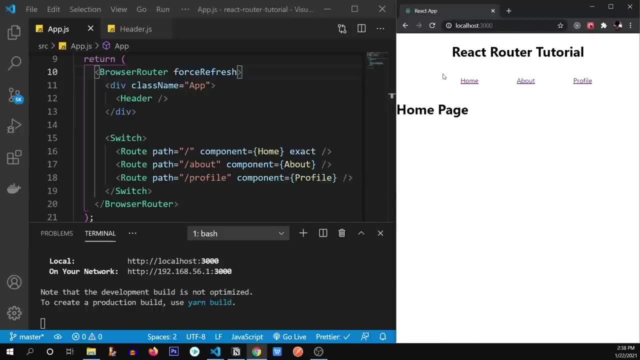 now It's providing the force refresh forcefully our app to re render everything, So you can use force refresh for that, which I don't think anyone needs to use. Also, if you want to confirm every time a user goes to another route, for example, if I click on 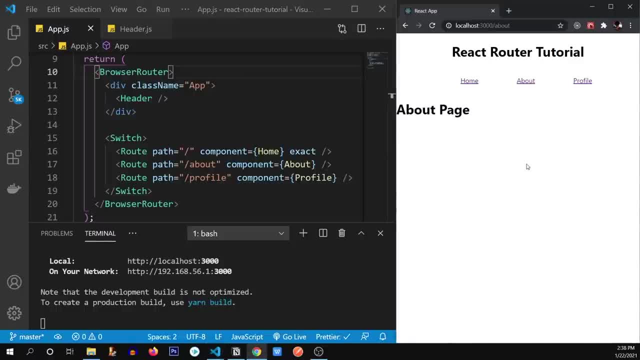 about. you need to confirm it by some prompt or by some displaying some model. what you can use is called get user confirmation. you can type get user confirmation And then inside of this you can write a custom message to be displays whenever the route changes. So 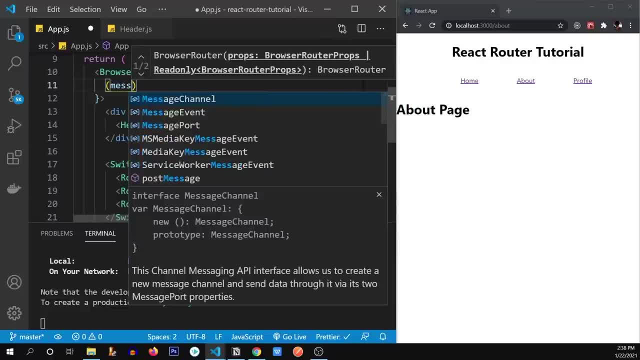 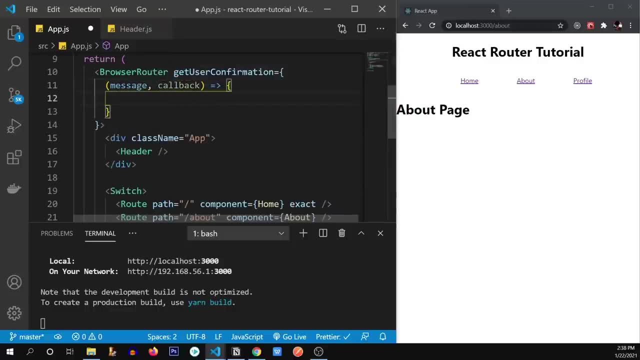 I'm going to write a function inside of it by typing message, whoops, message, and it's going to take a callback is going to be an arrow function, So callback is going to be an arrow function. So callback is going to be an arrow function. 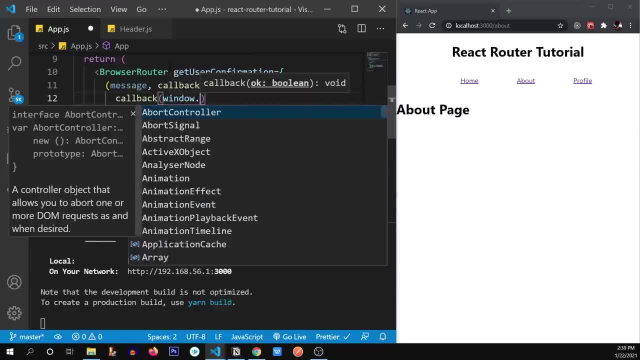 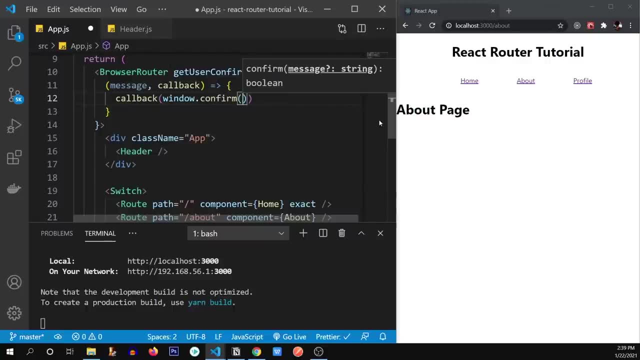 So callback is going to take window dot confirm And you can pass whatever component that you need to pass inside of it. Let's say, if you create a prompt, you can pass inside a prompt inside of it or a model, But I don't think this is used that much as well. So this is one of the features that 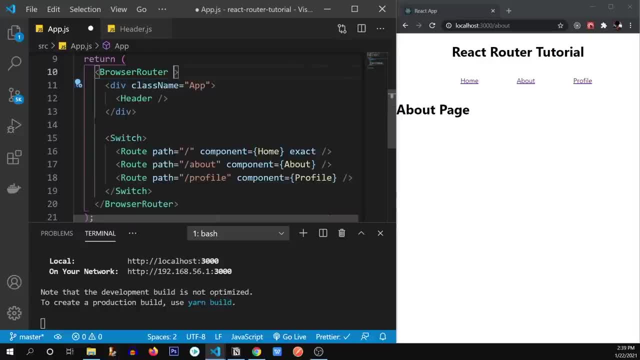 you can use in react autodom. So let's remove this. Yeah, All right, let's move forward. First of all, I want to show you how to use this. So let's remove this. So let's remove this. And. 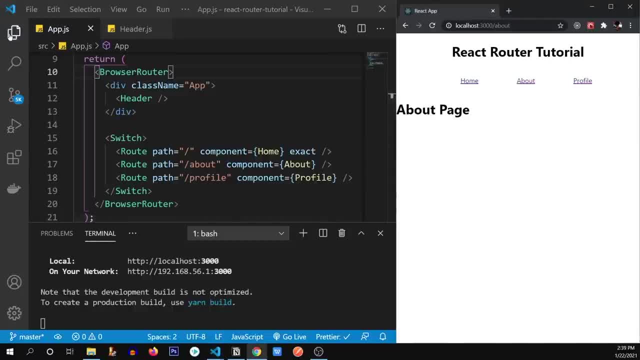 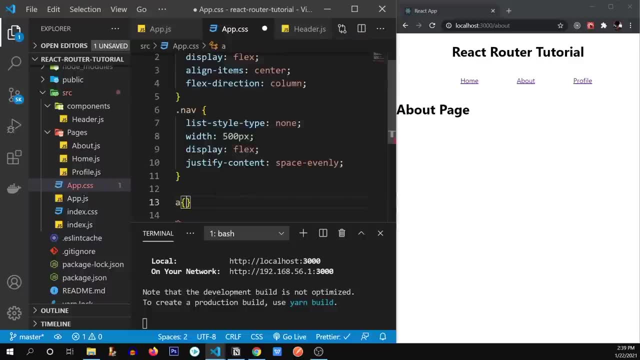 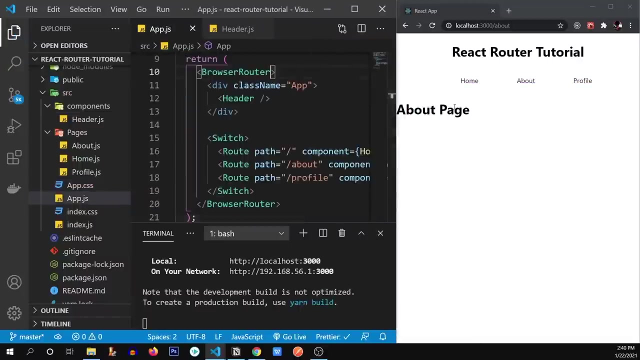 what I want to do is the let's remove these styles from the links. I don't want this style, So I'm going to go to app dot CSS And let's remove the styles by typing a removing text and decoration And color will be inherited. Yeah, fine, See, our pages are not that big right now, If you. 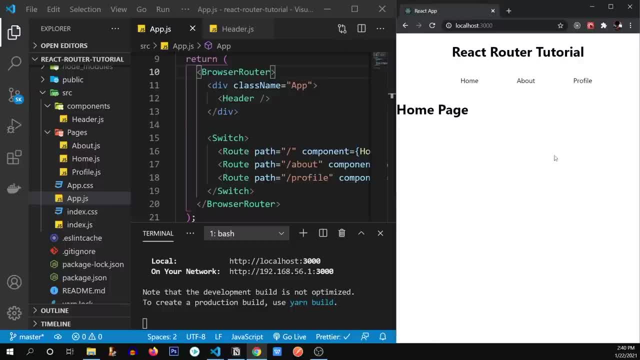 go to homepage, or if you go to profile page, it's. it's height is not that big right now, But let's say your, your page is so big that you need to scroll down. So whenever you change your route, what's going to happen? it's going to continue. the 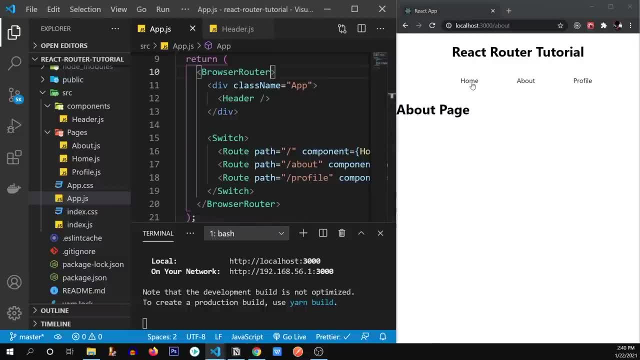 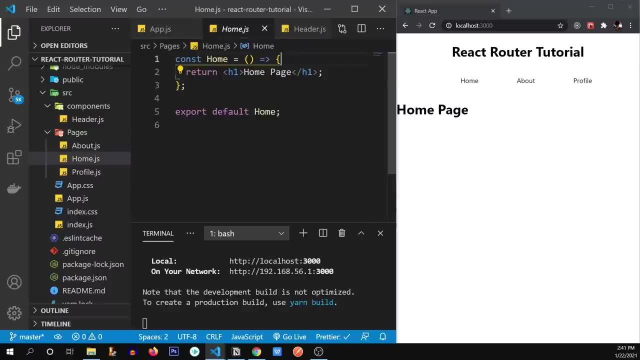 other page from the same position. So what you want to do in that case? whenever you go to a different component, you can type like this: let me just go over here to homepage, And you I can. what I can do is I can use use effect And inside of use effect I can type: 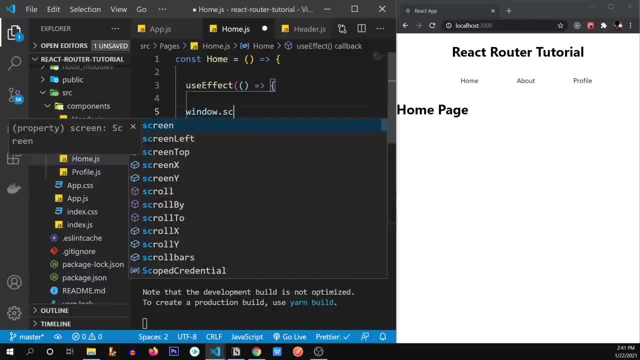 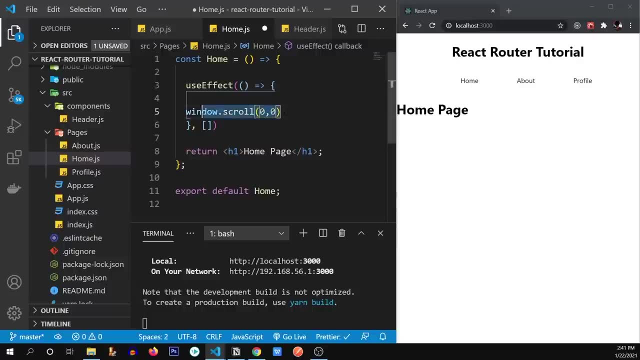 window dot scroll to zero, comma zero. So what it's going to do, it's going to continue the other page from the top and not the previous position. that page was when you were in the other component. So this is helpful, Okay. so next important thing is if, when we type to some other route that doesn't 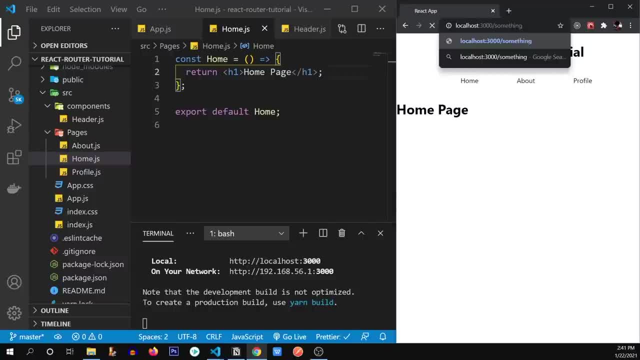 exist right now. let me say anything like something and enter. you can see there's nothing being displayed over here. we want something to display over here like 404 error page. not found something like that. So how can we display that over here? 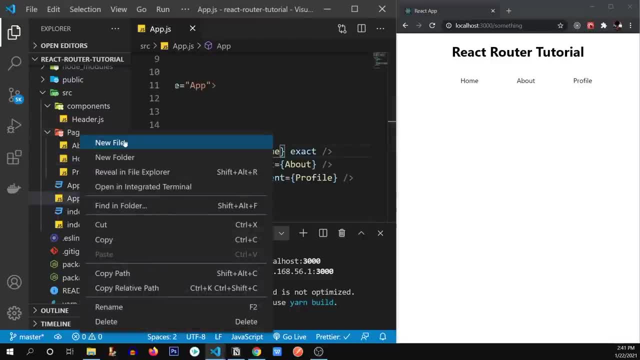 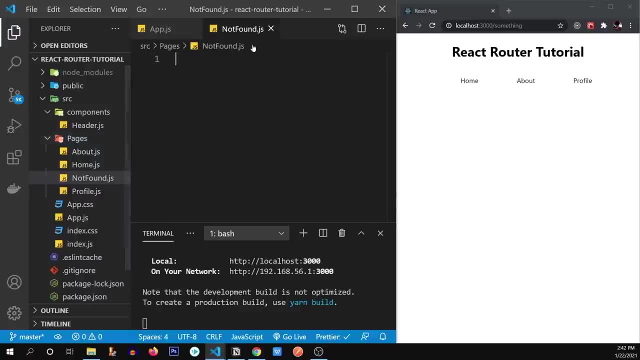 let me create a new page for that. I'm going to create a new page called not foundjs. All right, let's initialize this page. are a FCE, press Enter And I'm going to give it an h1 of 404- not found. 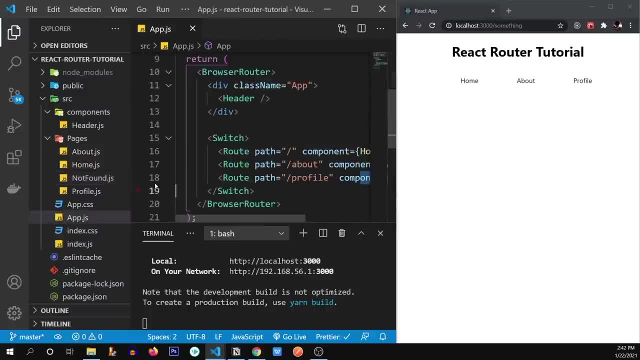 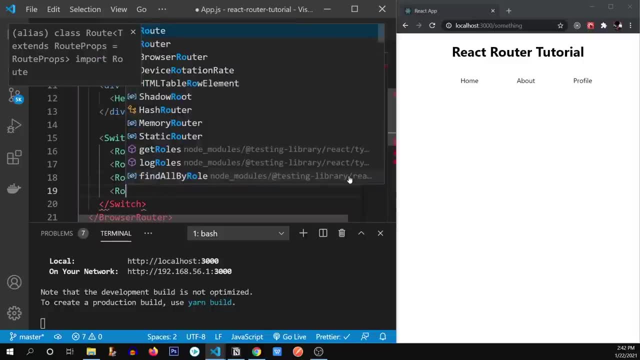 Let's save this Now. how can we, how can we use this Now? we need to go over here. let me close this. Yeah, we need to go over here. we need to create another route. If we did another route In this case, we're not going to give it any of the path, such as about: 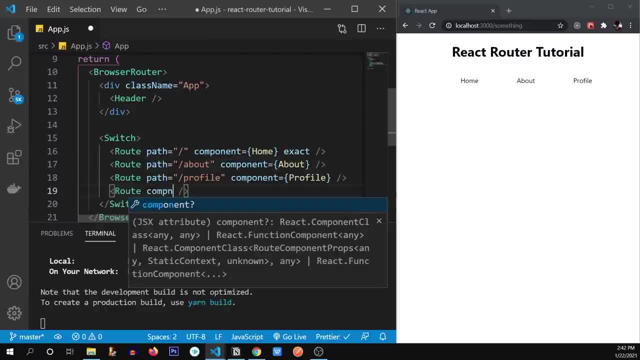 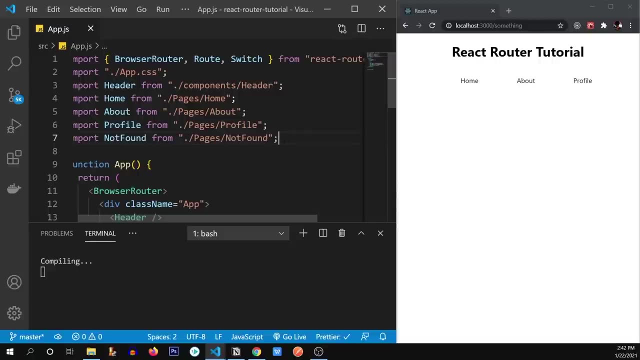 our profile or anything. we're just going to give it a component not found. I'm going to manually import it. Here we go. we've imported our not found page And here we go. the message is displayed successfully. If I go to somewhere else, 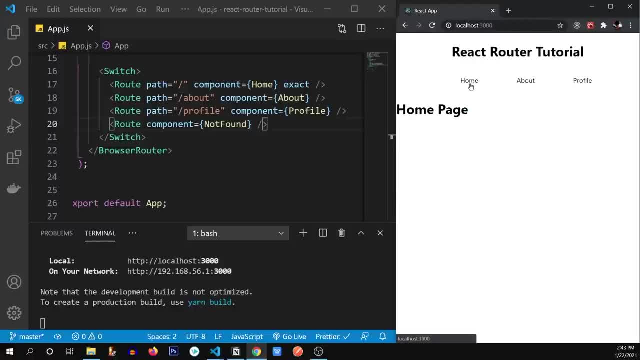 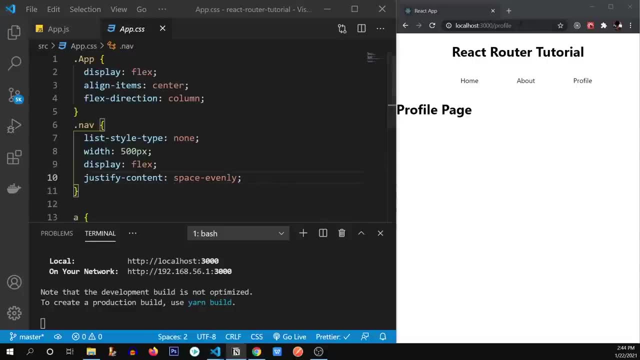 it's going to still display this message. If I go to a relevant page like home about your profile, it's not going to display any of the message. Alright, so let's move to the next thing, which is taking parameters from the URL. So let's say: if I want a page like something called post, 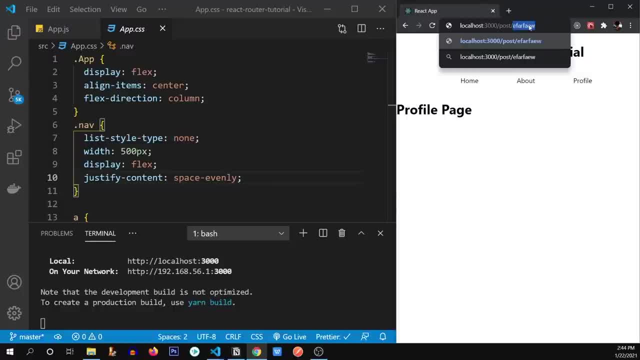 and we want some random post, So we want this random ID to be accessed by us. So what can we do over here? So currently it's going to show 404- not found. So let's create a new page for our post. 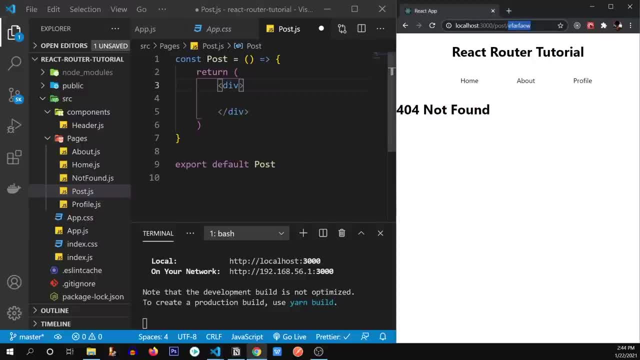 So what we want to do is one: we want to fetch this particular ID. So let me type: ID is and we're going to display the particular ID. I'm going to give it each two over here. Currently it's not going to display any. 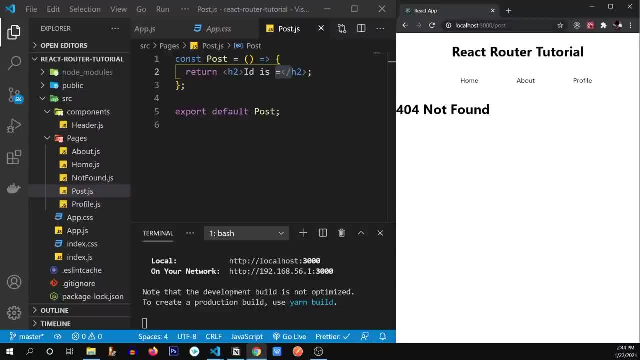 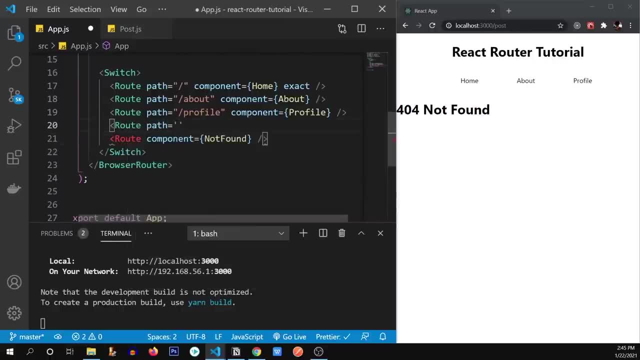 If I go to post: okay, we haven't created that out. Obviously we need to go to app js and create another route. Here we go. We have created this path successfully. Now you can see it's showing us ID is equals, which we can't do anything If we just slash, type anything. 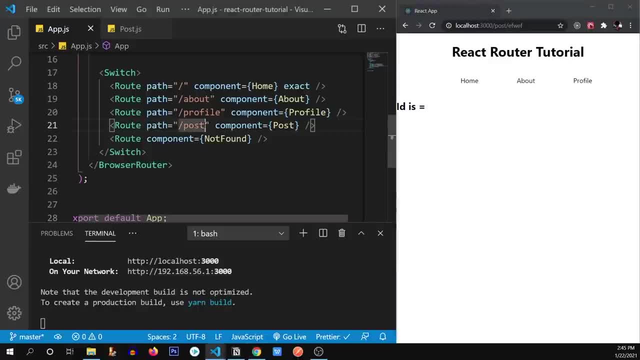 it's gonna know it's not going to display anything. So what we need to do- now we're going to do- is slash ID. So now it's going to take a random ID from us. So if I go to post now, it's going to display not. 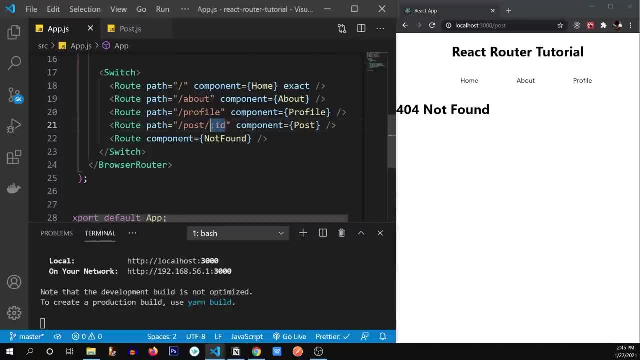 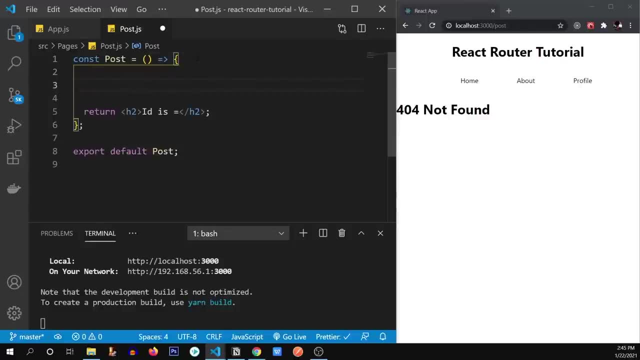 found, because that page doesn't want needs to have an ID to display. So let's go back to our page And now we're going to use our first hook, which is called use params. Or we can use a match as well. Let me just display, Let me just demonstrate it with the match first. So we're. 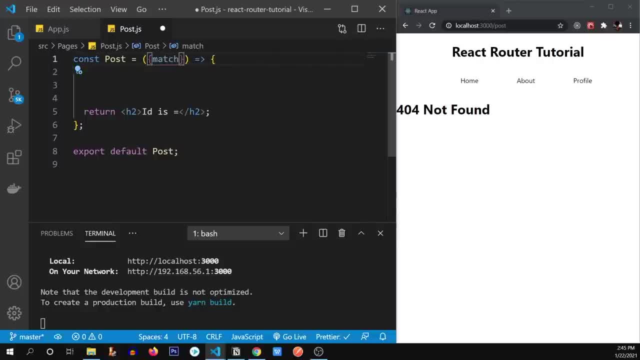 going to go over here, do destructure the match from here And now what we're going to do is we're gonna go over here and type match dot params And what? what was the name of the param? it was ID. let's save this And let's check this out Now. 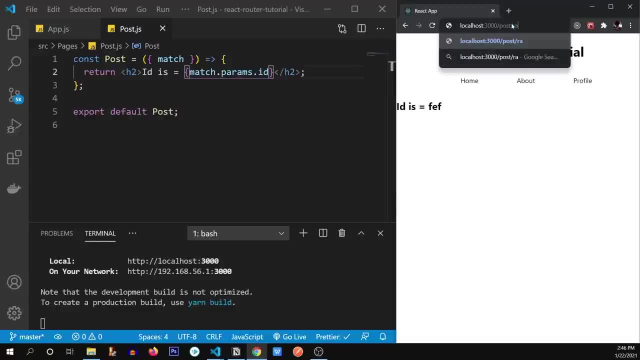 here we go. If I give this, let me type random over here and presenter: you can see the ID is generated and it's displayed over here. I mean it's not generated, we have provided it, but it's displayed over here. And now we're going to go over here and type match dot params. And now 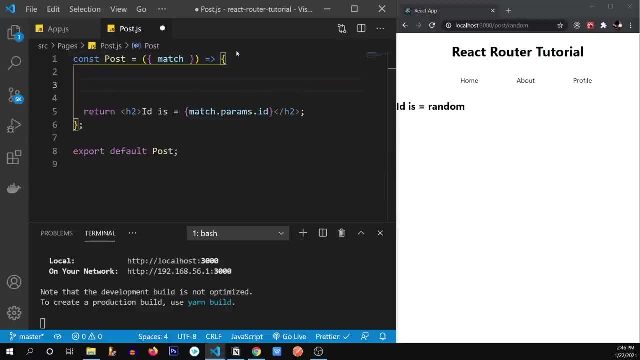 here we go. If I give this, let me check this out. Or we can just save this, let me check this out, And now here we go. If I give this, let me check this out, And now yeah. so what's the other other way to do this? The other way to do this is using us params. 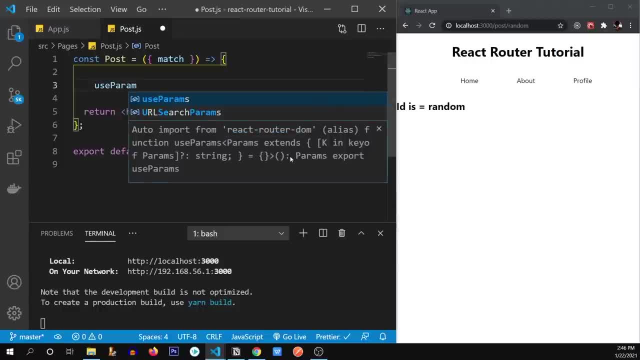 hook which is provided to us by react router DOM. So I'm going to click over here And you can see it has auto imported from reactor at home. Now we don't need this. I'm going to get rid of this. I'm going to use us params. Let's first log this us params. Let's see what do we. 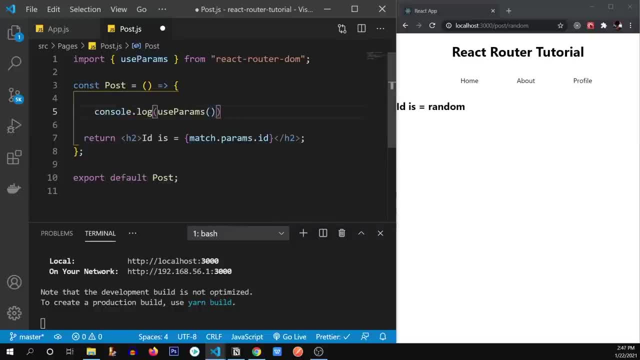 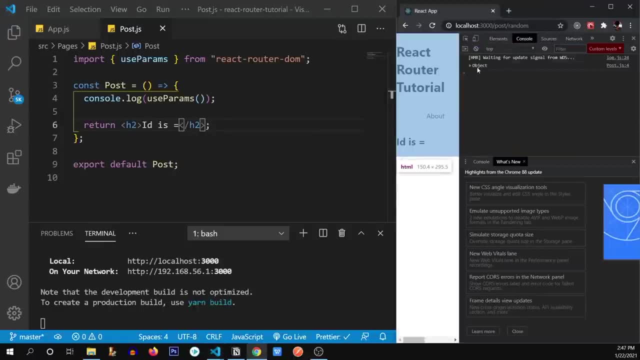 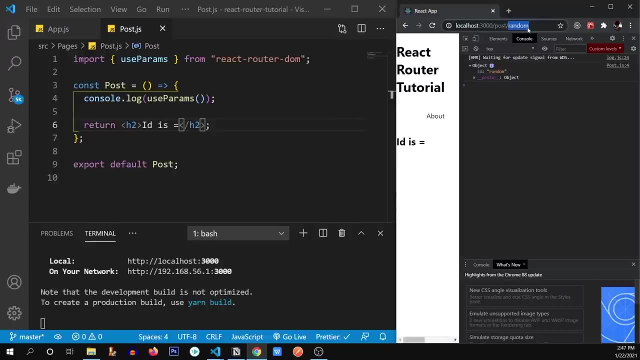 get inside of this. I'm going to remove this now So it doesn't give error. Alright, let's see log this, use params and inspect this. you get an object And this object has something called ID inside of it, which is the ID that we have passed over here. Let me type something and press. 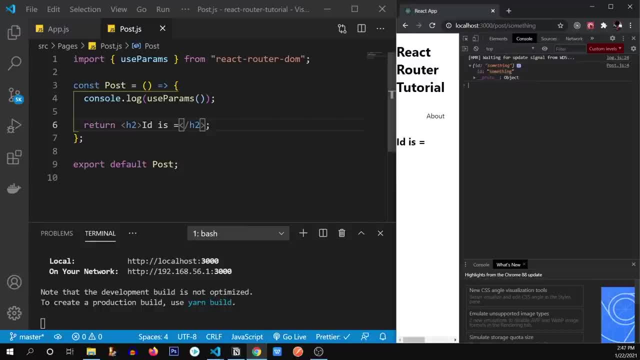 Here we go. It has given us another object with ID of something, So now we're going to use this use params. I'm going to type const Id equals use params And we're going to destructure this ID inside of the use params. So we have taken out this ID And we can just use this ID over here. 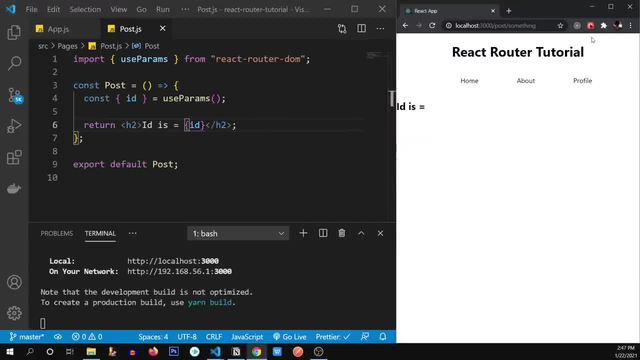 Now Let's save this. Let's check. here we go something. Let me give it a random number And here's our ID displayed successfully. So this is how you can fetch the ID from the URL. Now let's say we need to use a. we don't want to change our route, But we still need to use the variables from the URL. 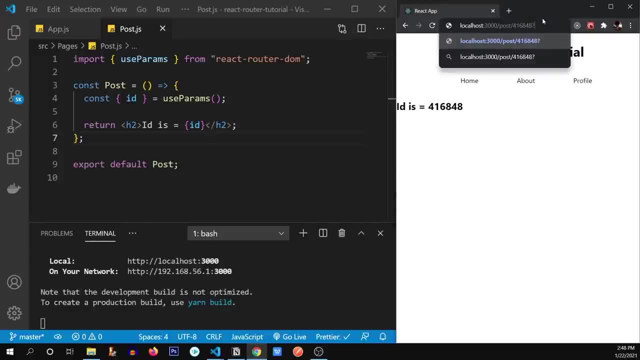 For example, if I type question mark and I, let's say I type name equals push. Let's say, we want this name, this name, how can we fetch this from the URL? Is there any other way? So we're going to. 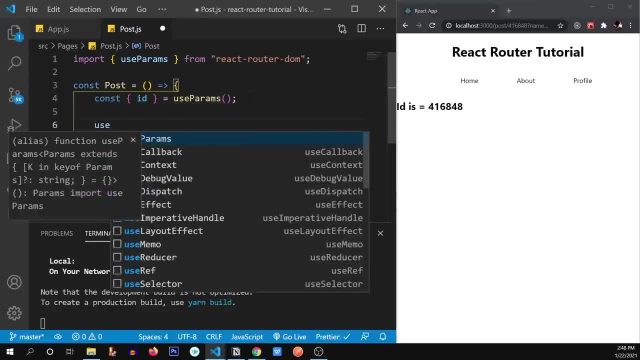 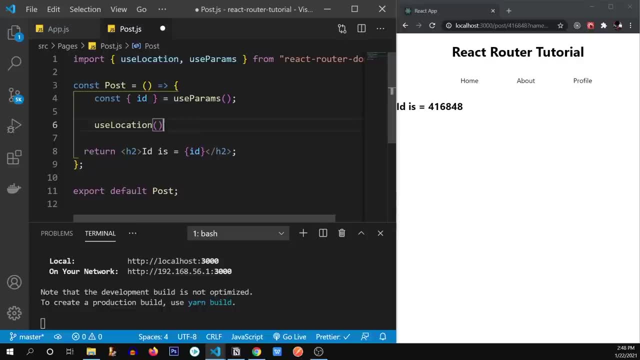 use our second hook called use location, use location And it's also provided to us by React router DOM, So we're going to type use location over here. let me just log this use location first and check what do we get inside of this? 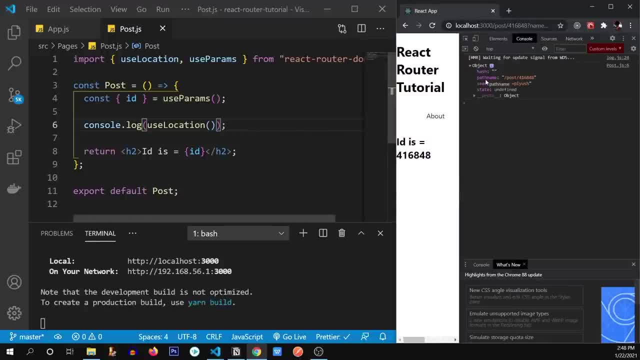 Let's go to inspect. We get an object, So what does this object has? it has a path name And it has a search with the value of name. equals push. Let me type something else: First equals push, And we can type. and last equals agarwal, which is my name. So yeah, 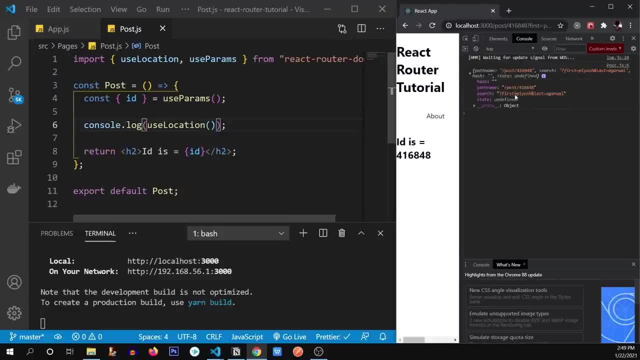 let's see Now. the value of search has changed to first equals tuition. last record: Agarwal. Now how do we fix these first and last variables from this search? you know, variable search object. So what I'm going to do now. so we're going to use an inbuilt API for something. Let me just go and go ahead and ruin some K tone. Let's go ahead and rewrite the technical information and check the technology that we have inside of K tone. Let's create the task that we have inside of K tone. So now I'm going to have a click. We're going to click, do. 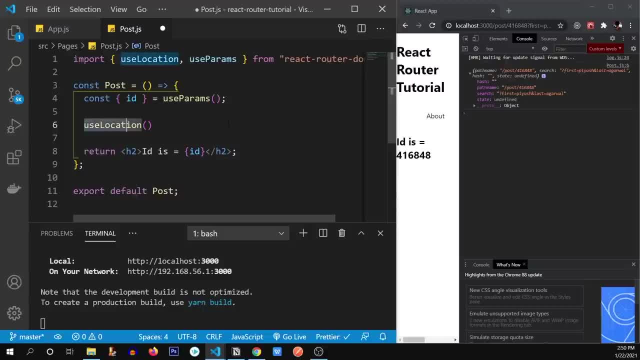 use an inbuilt API from the browser called URL search params. So I'm going to select it And I'm going to type URL search params And I'm going to create an object out of it, So I'm going to type new URL search params. And what do we want inside of this use location? we want this search, So 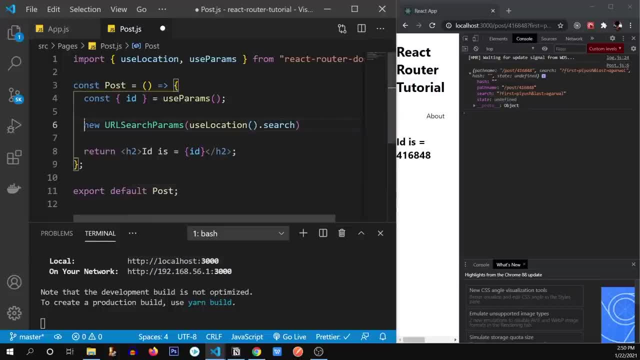 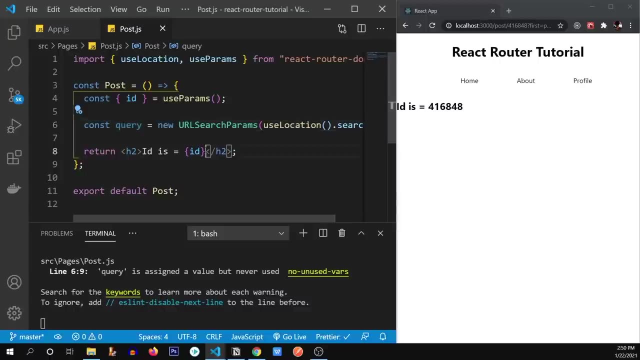 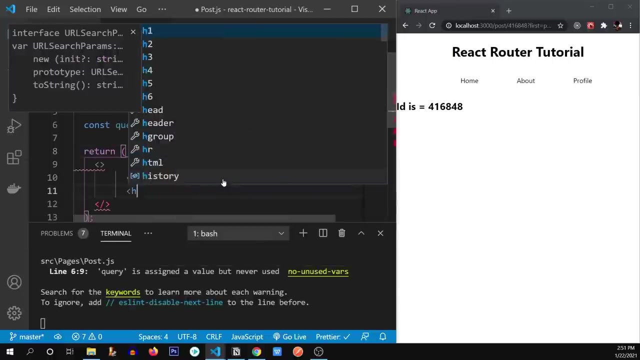 let's type search. Alright, let's take it in some variable. Let me type const: query equals new URL search params. Here we go. So how do we take out the stuff from this query? So let me just go over here and h2.. And we need to use the first and the last. So let's first extract the first one. So 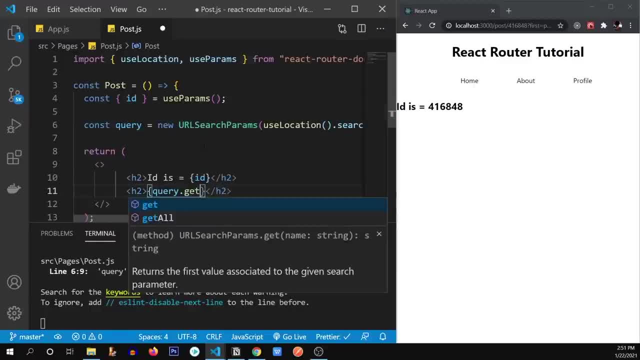 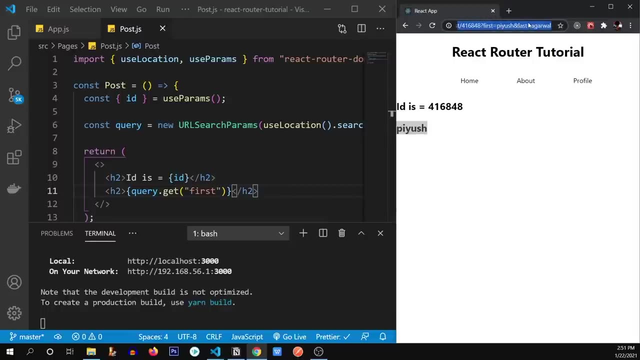 query dot get, And in the bracket we need to, we need to write the variable that we need to fetch from the URL. So I'm going to type first and save this. Let's see what happens. Okay, here we go. we get the puge from here, from the first, and let's fetch the last as well. 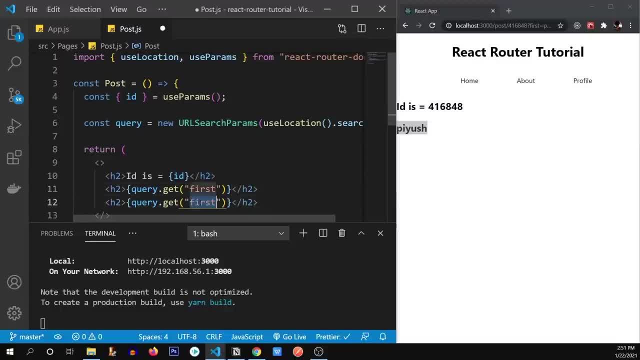 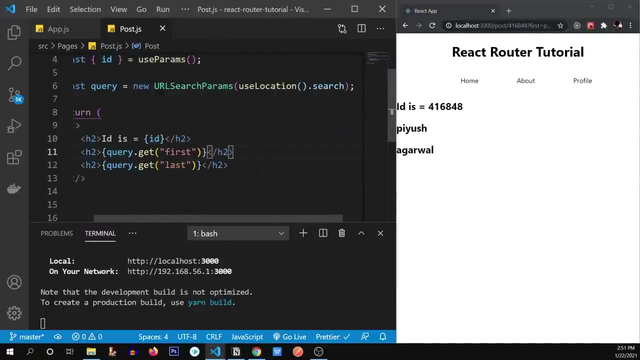 Last, Here we go. So we can type n number of queries inside of this URL And we can fetch them by using this method: use locations hook. So that's pretty cool. Now let's see. let's suppose you have a login feature in your app And you want user to access the profile. 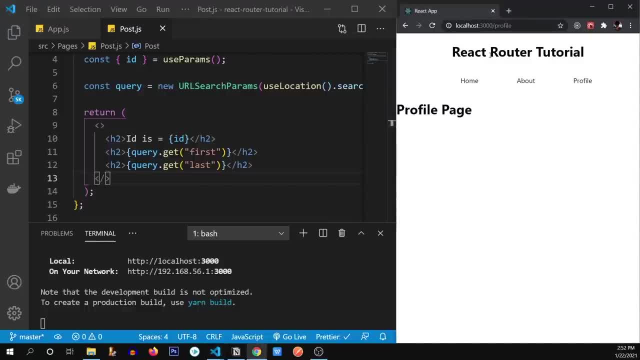 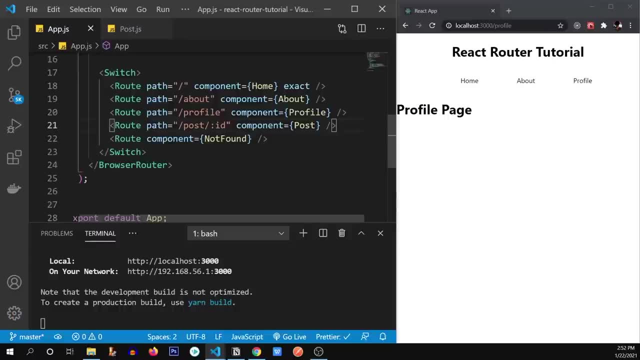 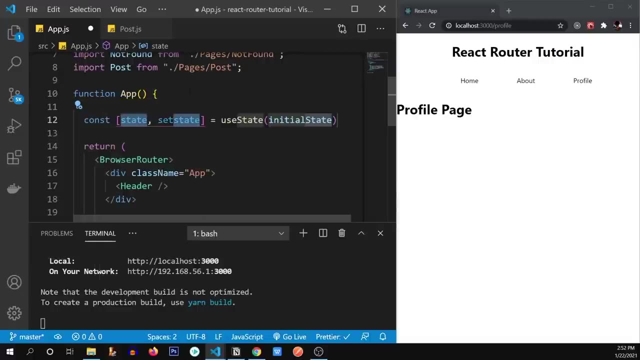 only if that user logs in into your app. So how are we going to modify our react outer DOM according to that? Let's find out. We're going to go to app js And we're going to create a new state, Let's say login. Let me import the user state from react. Here we go. So 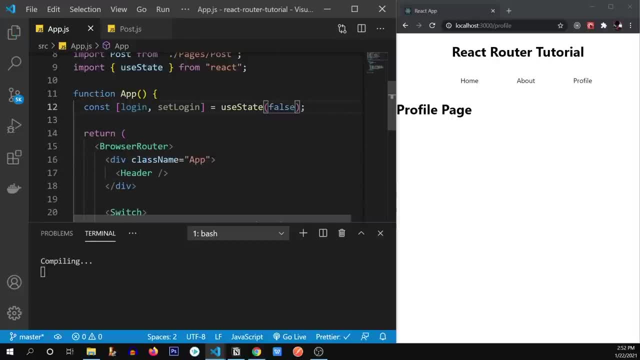 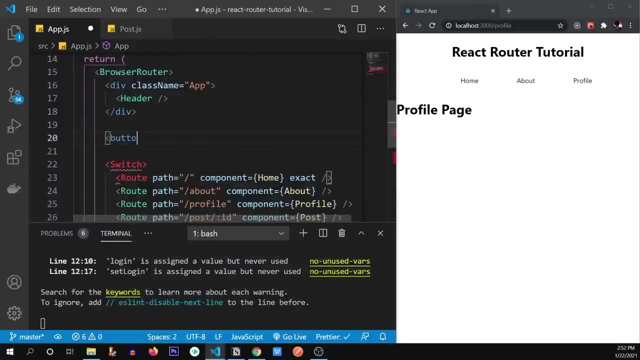 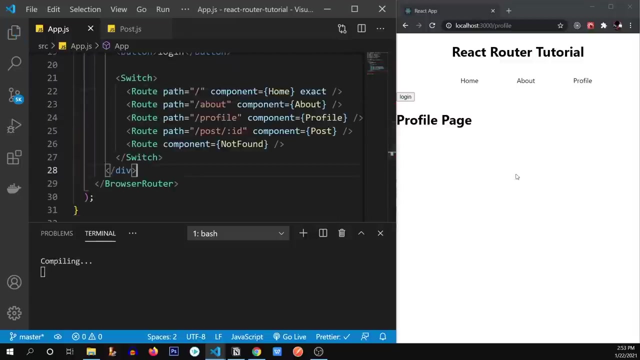 by default, login will be false. Login will have false value because we are not logged in now. And let me, let me just create a button over here to log in. But we're going to go over here. Let me just take this div and put it over here so that everything is centered. Yes, 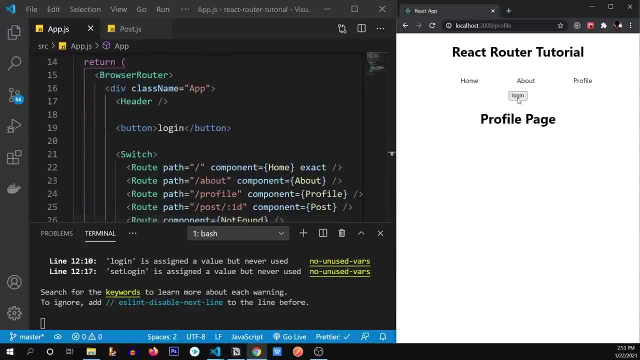 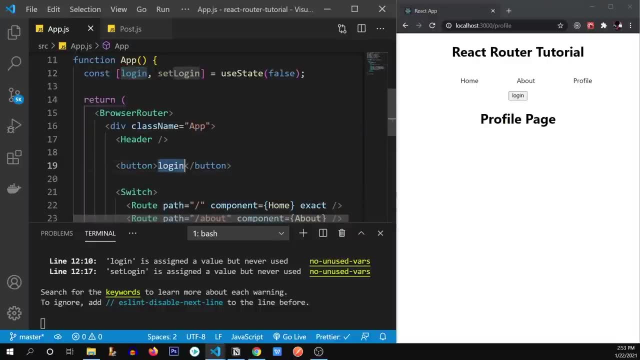 it's centered. So what I want is, when I tap on this login, we're going to simulate a login feature by making this login as true and it's going to display log out then. So on click, what it should do, it should set login as the opposite value. So if it's true, 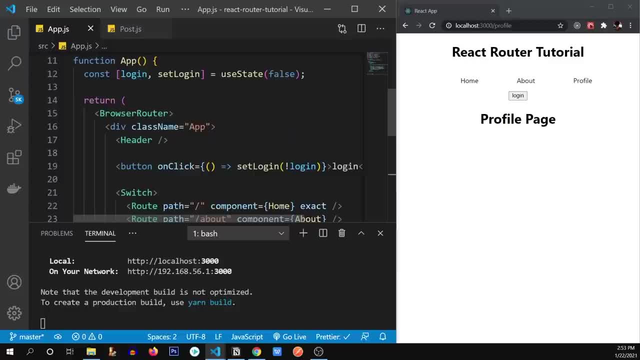 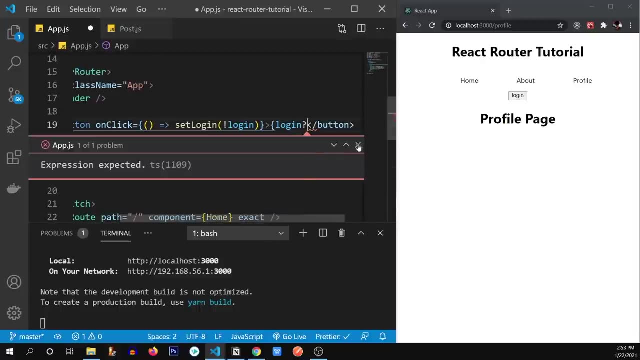 it's going to be false. If it's false, it's going to be true. Also, what I'll display over here is if login is true. if, which means if user has successfully logged in, then it should display: Whoa, what's happening? Yeah, then it should display log out. Otherwise, it should display 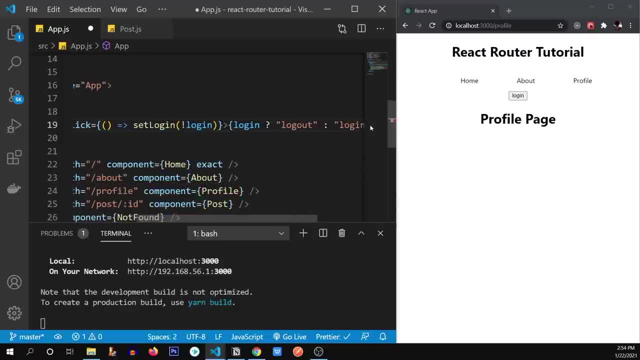 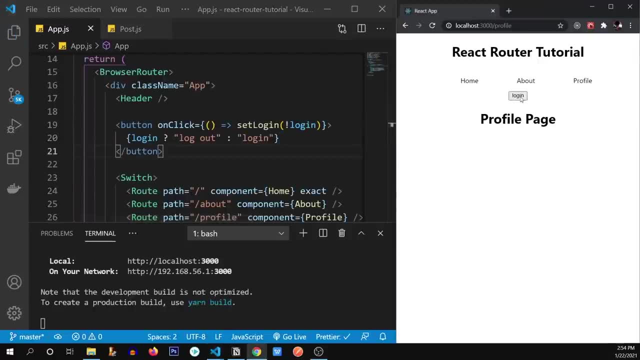 login, Let's save this and let's see if it's working or not. Okay, it's working, fine, So what do we want to do over here? if our user is not logged in, he's not going to be able to access the profile page and he's going to be redirected to the 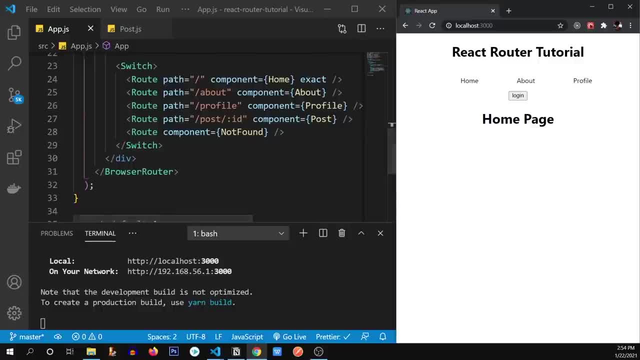 homepage. So how can we achieve that? we're going to use something called redirect from react outer DOM, So let's remove this component from here. How I'm going to do this is here. we're going to make the the child component of this route, So let's check this over here, If login. 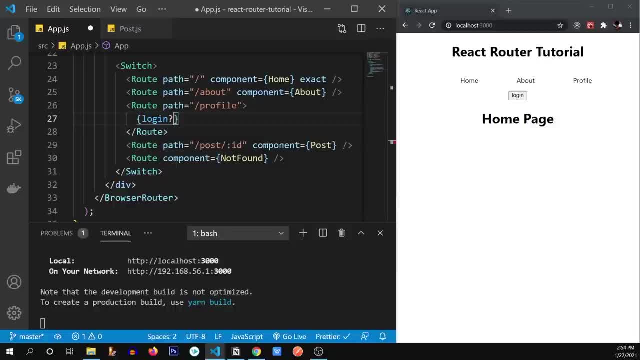 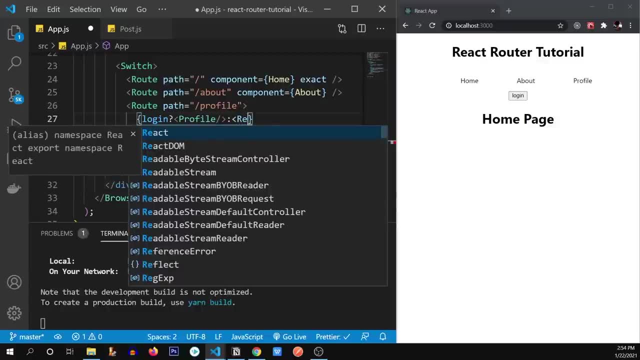 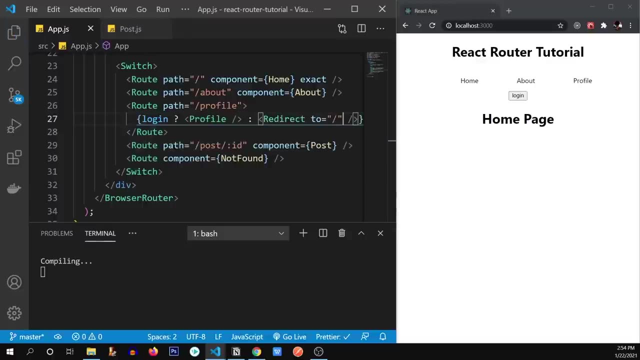 is true, if login is true, then it's going to be able to access the profile page, So profile. otherwise it's going to be redirected, So redirect. Well, will it be redirected to homepage? Here we go. All right, let's try clicking on our profile page. let me go to about page And let's 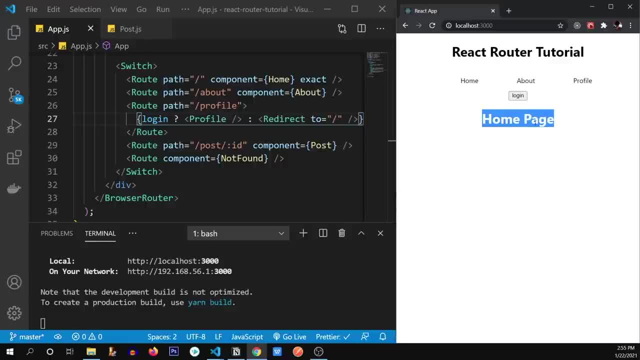 click on profile page, you can see we have been redirected to homepage. we can't access the profile page, But the moment we press login and let's go to profile page Now, now we're able to access the profile page, So it has became a protected route for our app If I'm inside of this profile. 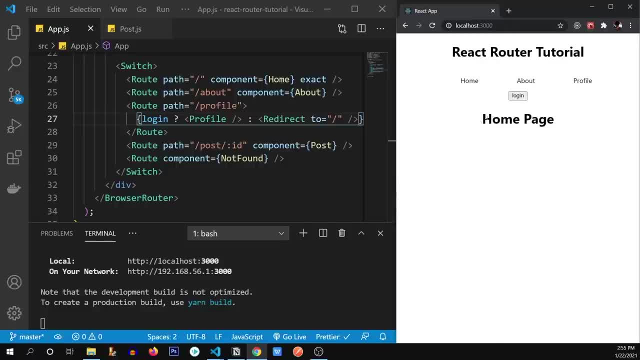 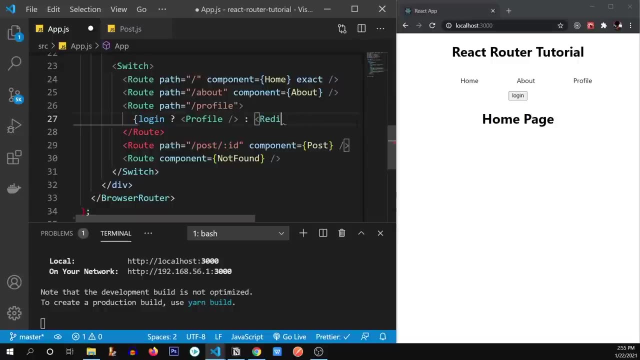 page and if I press logout- let's see what happens- It's going to redirect us back to the homepage. Now there's another way of doing this. Let me show you we can use something called use history- use history hook. So let me just type this over here: I'm going to remove all of this redirect. 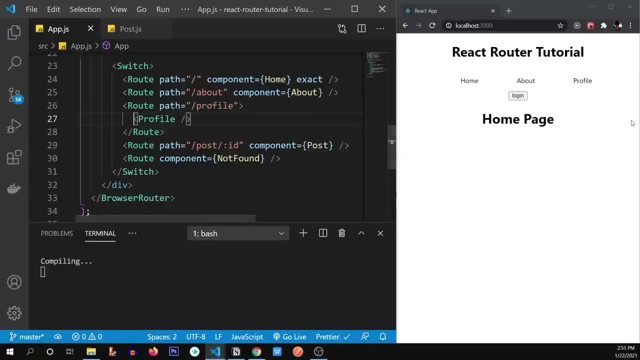 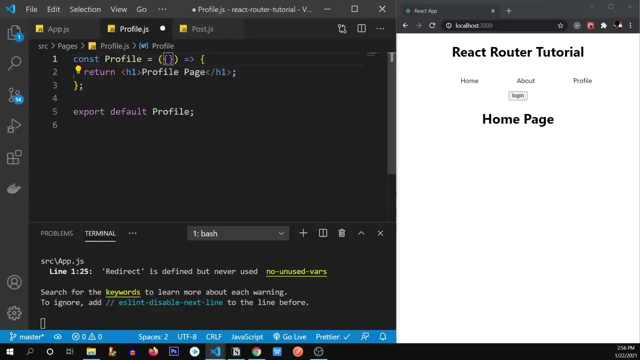 and make it a normal route. now It's working normally now without login. Alright, so I'm going to. what I'm going to do is I'm going to send the login as a parameter inside of this. So send the login as a params that go to profile and destructure the login out of here. Here we go And 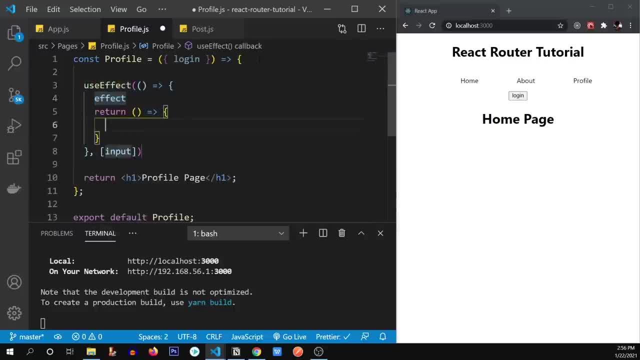 let's create a use effect. So use effect runs whenever our app is initialized first time. So I'm going to take the history out of the use history hook. So let's type use history And I'm going to assign it to const history. 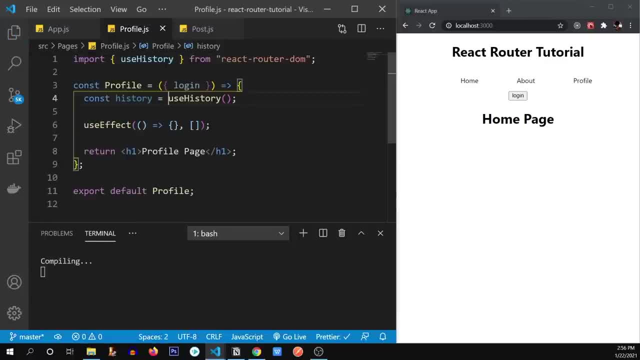 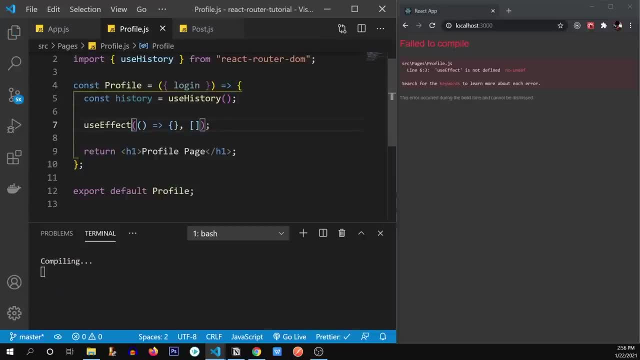 variable. All right, It has auto imported from react autodom. What happened? Okay, we haven't imported the use effect. Here we go, Alright. so what do we need to type inside of the use effect? we need to check if the user is. 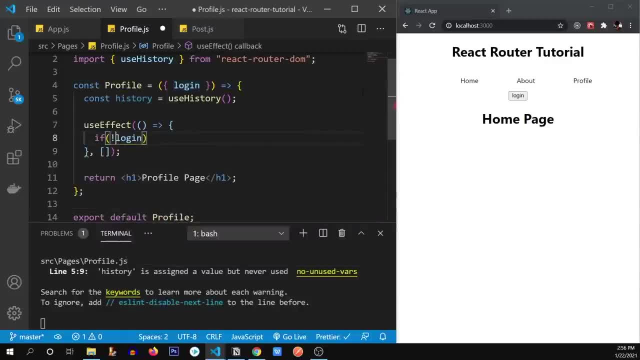 logged in, or if the user is not logged in, what are we going to do? if he's not logged in, then we will use history dot push. it's going to push this path to our URL. So it's going to push to the slash page, which is: 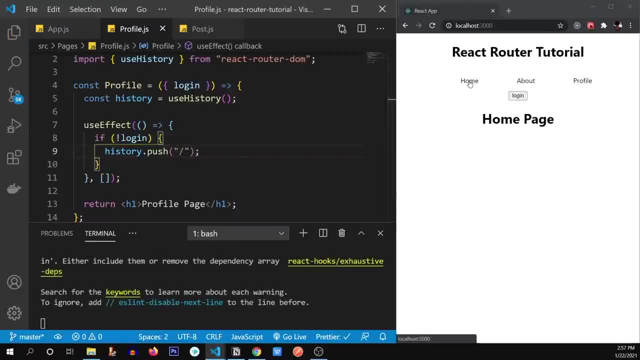 our homepage. So let's try this out. I'm at the homepage. let's go to profile page. I'm not able to access the profile page Now. Let's log in And let's go to profile page. Here we go. We're successfully in the profile page. 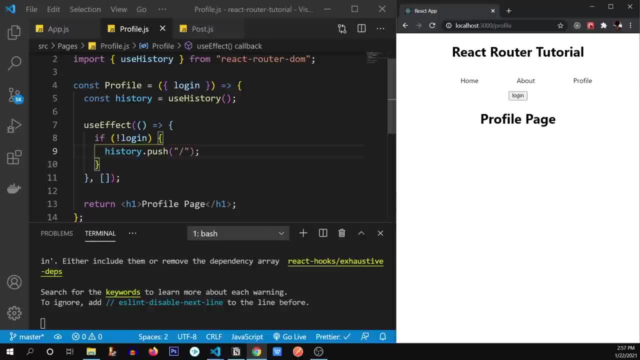 And let's log out now. Whoa, what happened? I think I have missed some. Yeah, okay, So if we want it to run whenever the login variable changes, so I'm going to provide login over here and history we're going to provide. 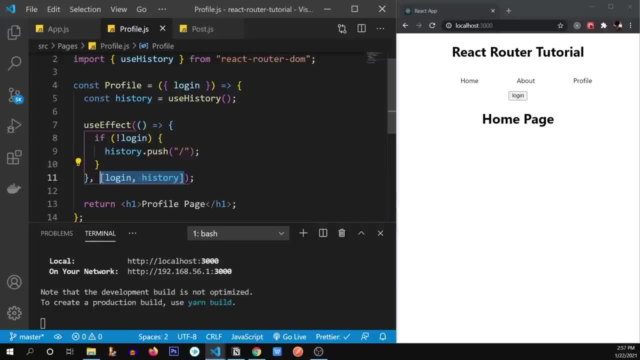 these two dependencies inside of the use effect. whenever these two dependencies are going to change, it's going to fire off this function Again. we're going to go to profile. it's not going there. I'm going to type, I'm going to click on login. What am I? 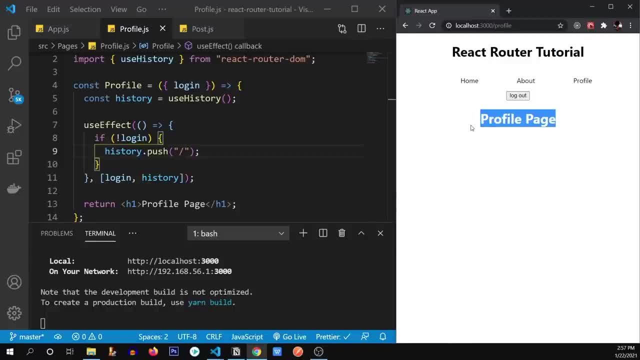 saying today: Okay, so let's go to profile. Now, Here we go. We're able to access the profile page. Let's log out, Here we go. We're back at the homepage. If we want to go to about page about, let's say: if the user is not logged in, he's. 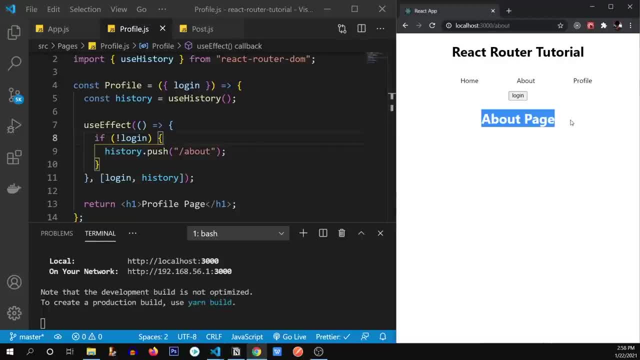 going to go to about page. if I click on profile, see, it redirects us to about page. but if you're logged in, we go to profile page. So I hope you all understood This feature of react autodom. Let's move to the next feature. So let's discuss how can we create a nested route inside of a 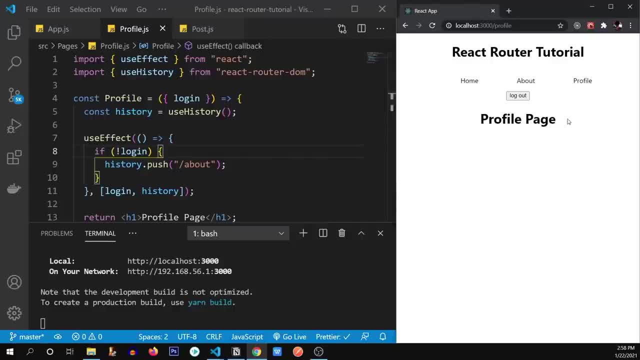 particular page, For example, if inside of the profile page I want to create two routes with the name of, let's say, view profile and edit profile, And I don't want those two routes to affect our whole react router system, We only want them to. 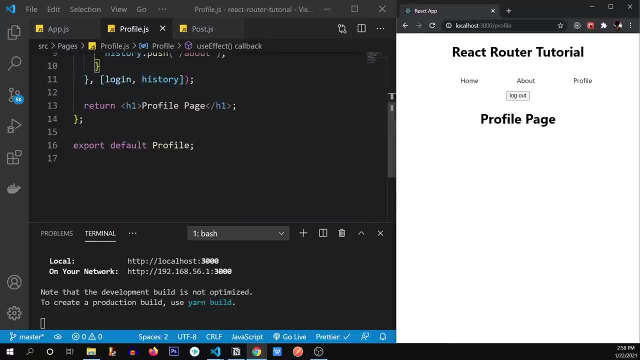 work inside of this profile page. So let's create two new routes over here. I'm going to remove this. Let me just put it inside of this round braces and then provide react fragments to these. Alright, let's move this. Yeah, so I'm going to create a nav bar inside of a profile page. 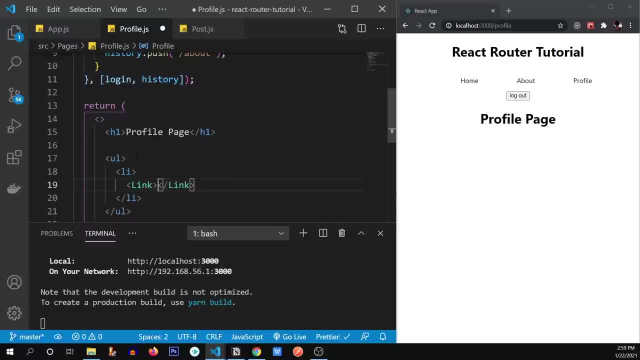 I'm going to create a link tag over here- Let's say view, And the other link tag is gonna have An edit, edit profile. let's say Also: we haven't created these view profile and earth profile components yet, So we also have to create those view. 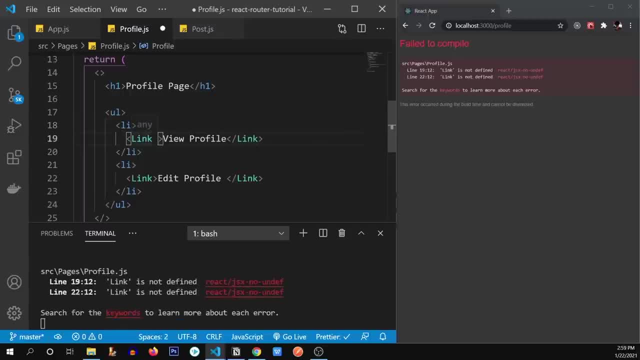 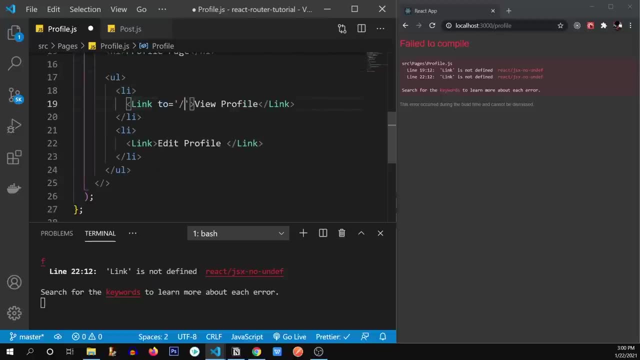 profile. We need to provide a to. It's going to go to 되. So, first of all, before doing all of this, let's create a route and the component first, so that we have these errors out of the way. So I'm going to go below this And, as usual, we're going to create. 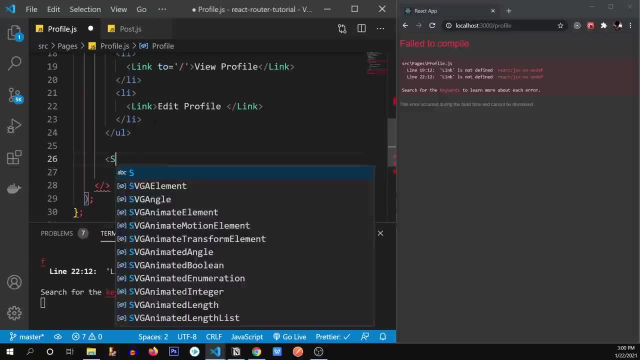 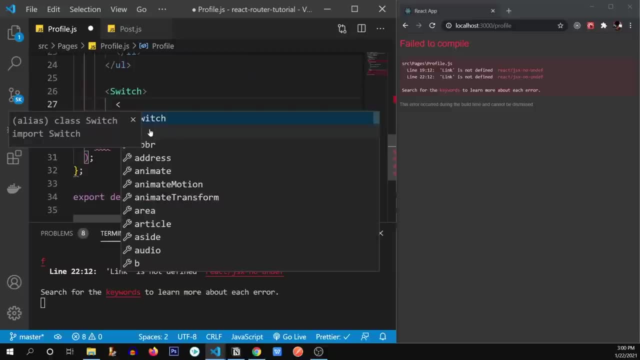 a switch, Whoops, switch. Let's see what has auto imported or not. Yes, it has. All right. we need to create two routes. Route one will have part of slash view profile, And it has. it's going to have some component which I'm going to create next, And the other one will. 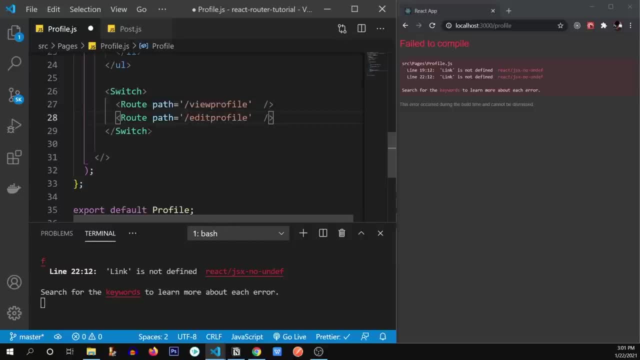 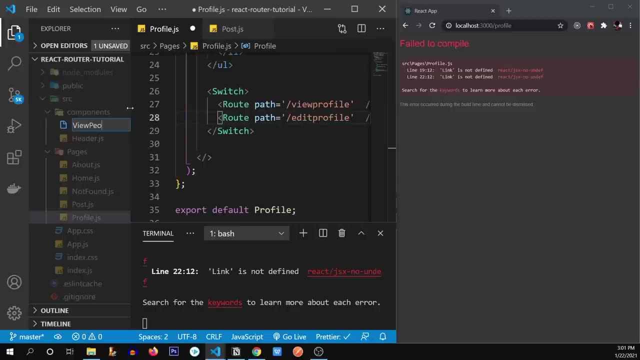 be the edit profile. Edit profile: Yeah, let's create those two components first. View profile dot j s. Okay, I made a spelling mistake. View profile dot j l. What the heck? P r o f i l e- Yes. 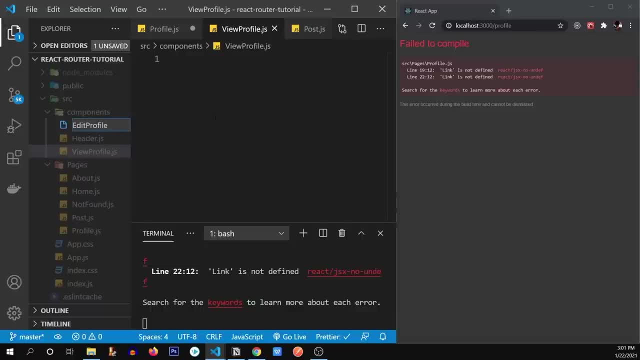 Edit profile: dot. whoops, dot j s. Yeah, let's create this r, a, f, c, e And I'm gonna give it a h two and view profile page. Okay, this component has been created and same with the edit profile page. Edit profile page. giving this h two as well. Yeah, Fine, Let's move on to the next. 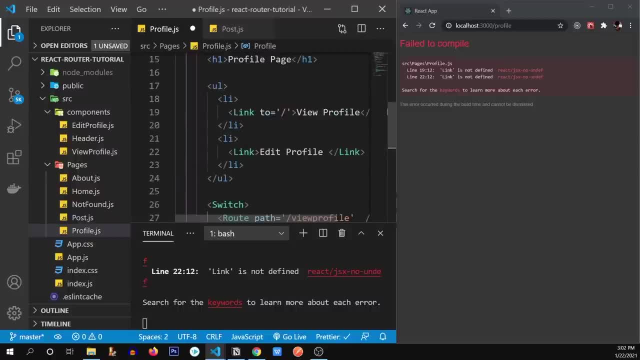 thing. Now we're going to go back to our profile page And over here we're going to go and give it a two to slash edit profile And this one to the view profile. Let's see if it works or not. route is not defined, Obviously. 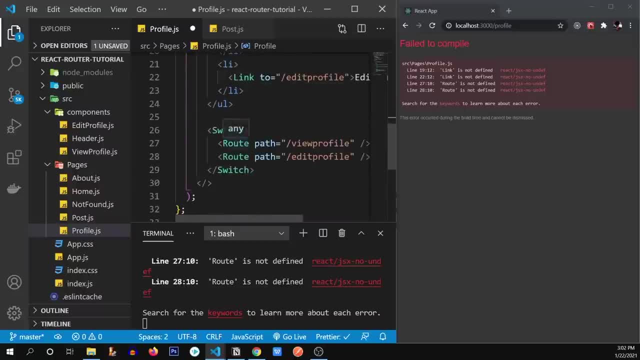 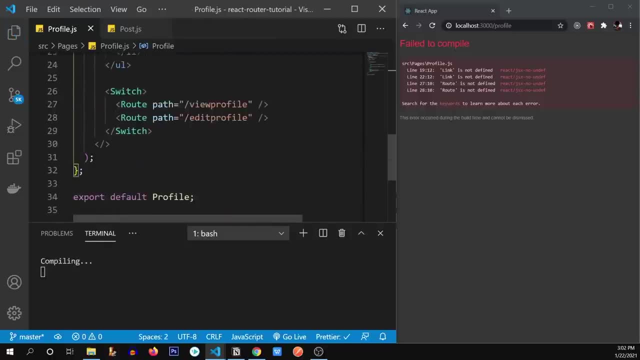 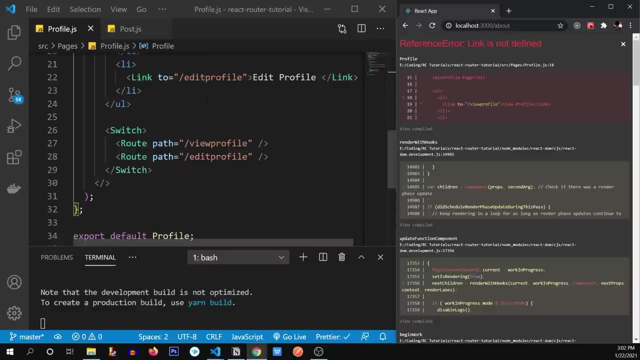 route and links are not defined yet, So I'm going to auto imported from the VS code With the help of VS code here. Here we go. All of these are important now. Alright, let's see what's the error over here. link is not defined. Link is defined, you can see. link is. 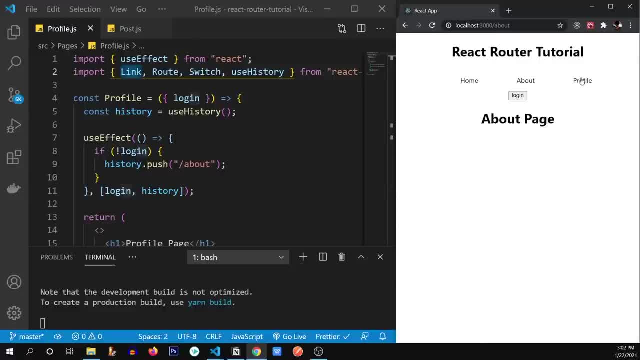 is defined over here. Let's maybe let me refresh this. Yeah, it's working fine. Let's go to the profile. Okay, we have to log in first. And let's go to profile. Okay, we have view profile and edit. 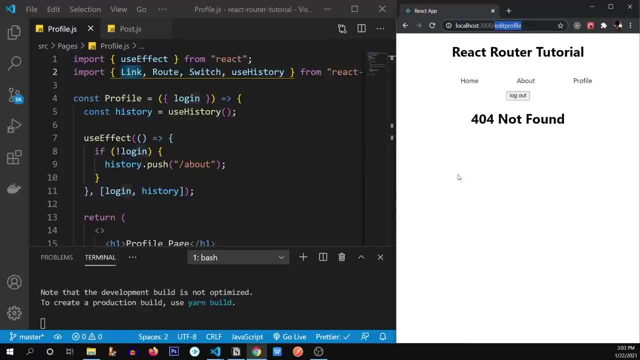 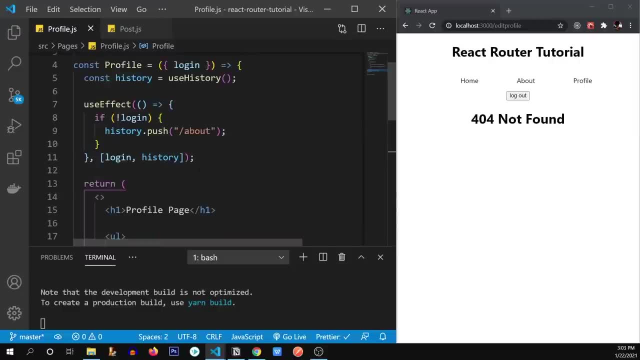 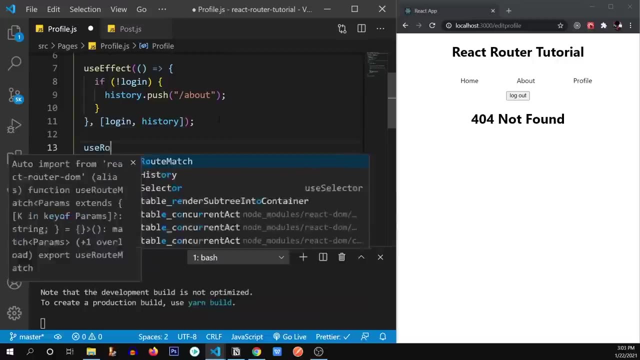 profile over here, But it's not working now. But why is it not working now? Because we have already created our routes over here. So what do we need to do? So what do we need to use now? Because we're going to use something called use route match hook. use route match. 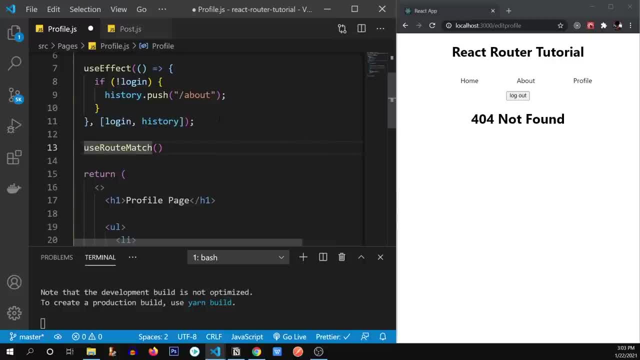 So this is the hook that we're gonna use to help us, you know, move on, nest the components inside of other component. So let me type const And I'm going to take out something called path and something called URL from inside of this thing. So let's see how can we use this path and 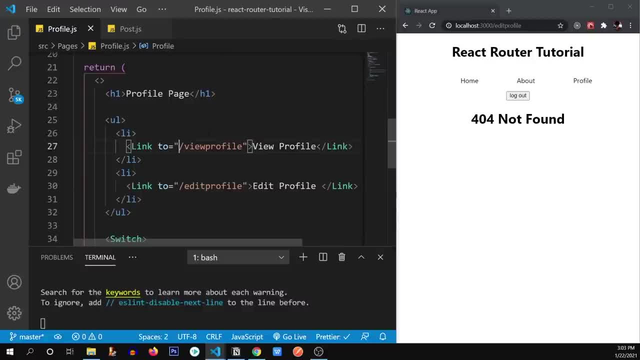 URL First of all we want to go to- we don't want to go to- view profile because it's taking us to slash Edit profile or slash view profile. we want to go, for example, if you're at the profile, we want to take the current URL and then append the view profile after it. So what I'm going to? 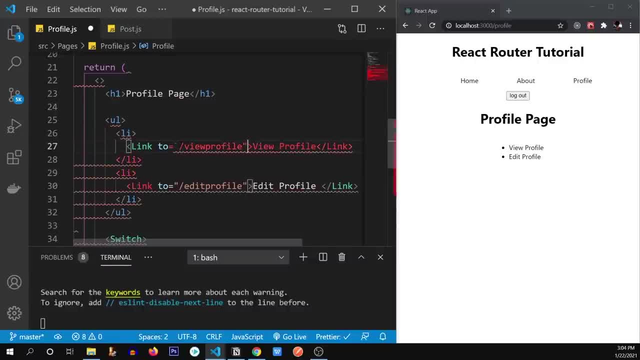 type over here. first of all, I'm going to remove this standard string tags and going to use back ticks, Oops like that. Okay, so now we need to provide a variable inside of it, So we're going to type URL, which will be URL. Yep, now it's going to work fine, And the same over. 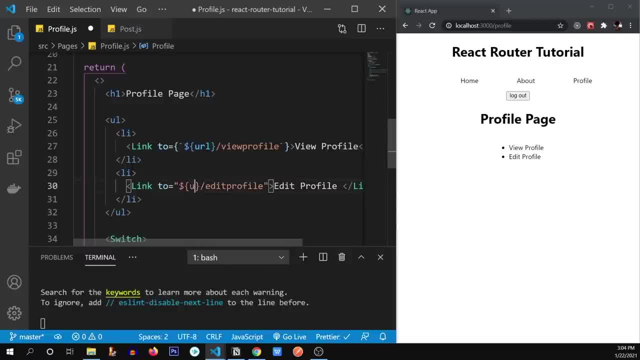 here URL, and I'm going to remove the string and give it a back tick, Just like that. So this is how it's going to work, And over here as well. Okay, we haven't given it the component prop, So it's going to work. And over here as well. Okay, we haven't given it the component prop, So it's. 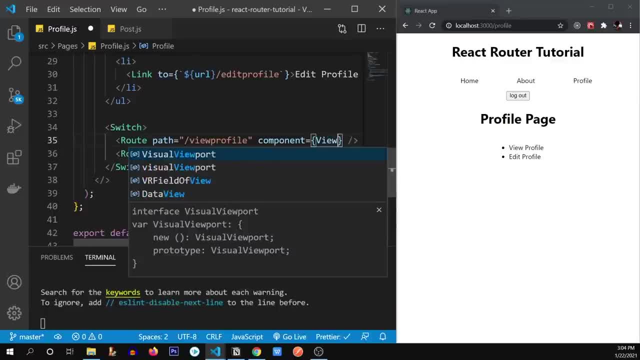 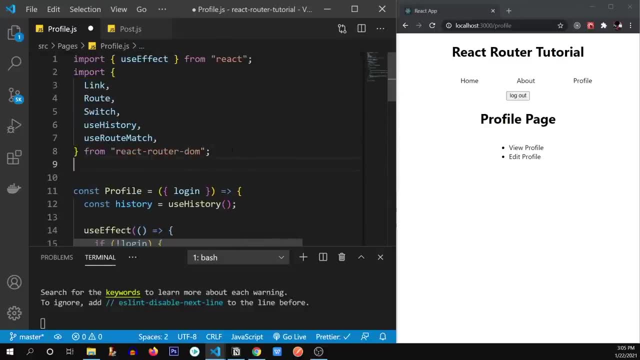 going to be view View profile so it's not auto importing. let me just import it over here. View profile from. have to go one step back and inside of the components and view profile. same with the Edit profile as well. Edit profile. it should work now.